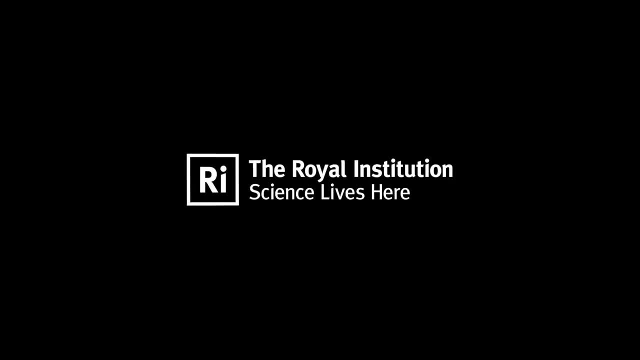 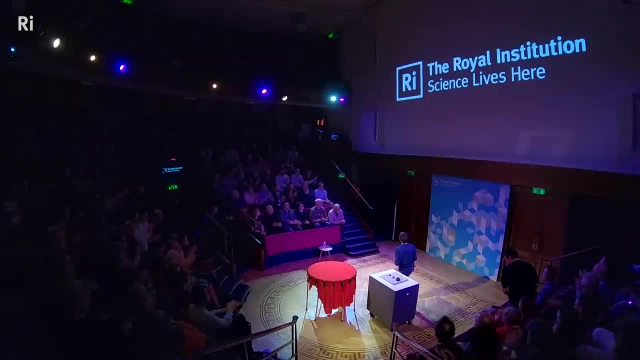 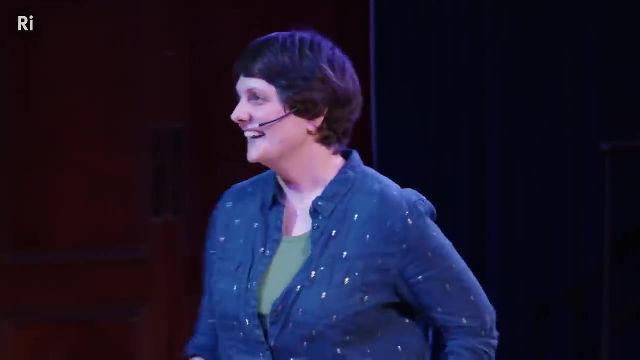 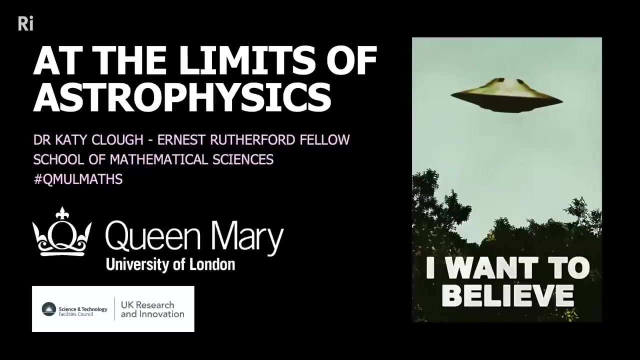 Hello, thank you, and thank you especially for the promotion to professor. I am sadly only a doctor, but, yes, I'm nevertheless very happy to be here this evening. So yeah, as Hasan said, I'm Dr Katie Clough, So I am an Ernest Rutherford Fellow at Queen Mary. 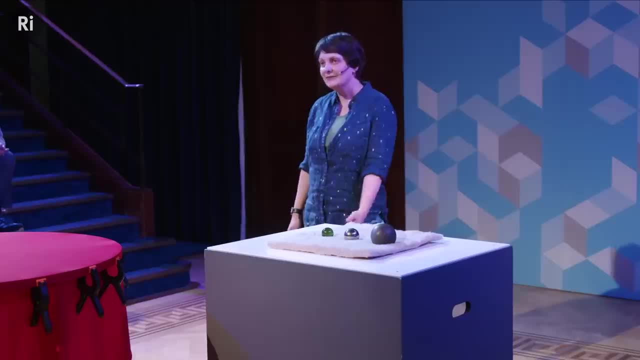 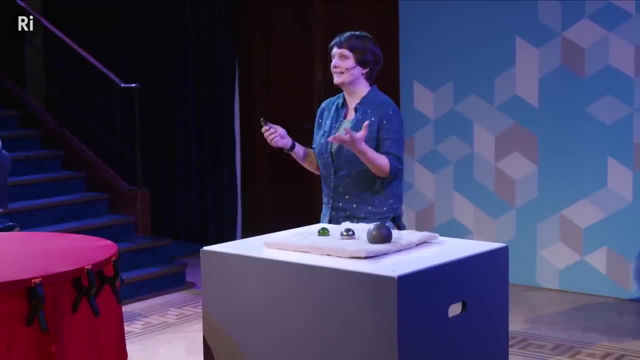 University of London, which is just down the road, And this evening I'm going to be telling you about the limits of astrophysics. That's what I promised to tell you. So the title: At the Limits of Astrophysics- so that's the title of my talk, but it's also a bit of a description. 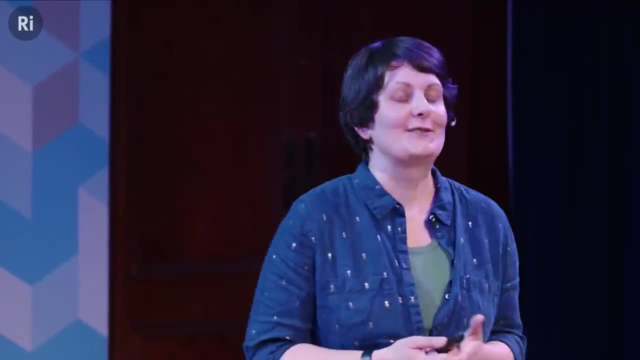 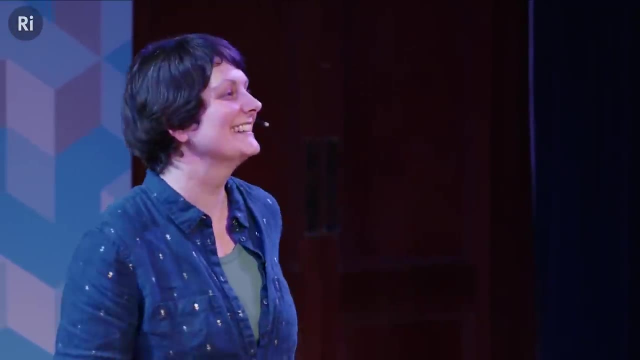 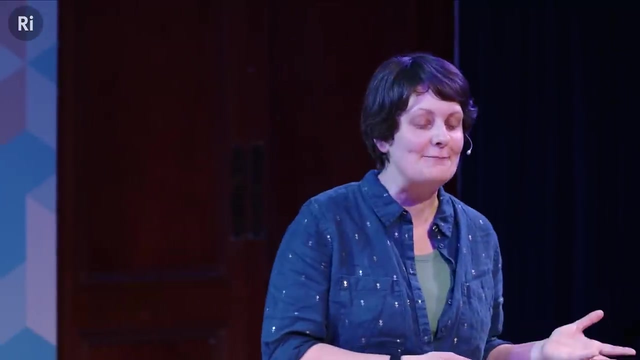 of me and my research, So you'll notice from my slide that I'm actually from the maths department at Queen Mary University. We've got some mathematicians in the audience And so actually all the mathematicians think I'm an astrophysicist. but all the people in the astronomy unit who are 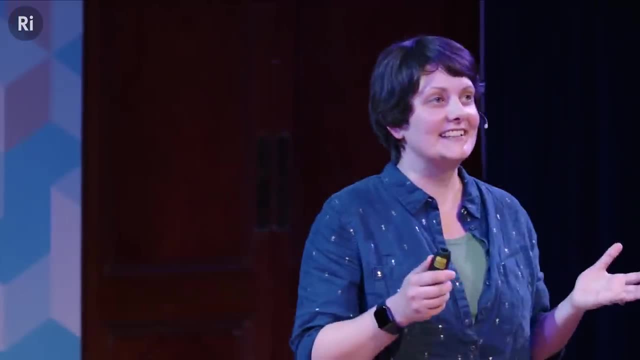 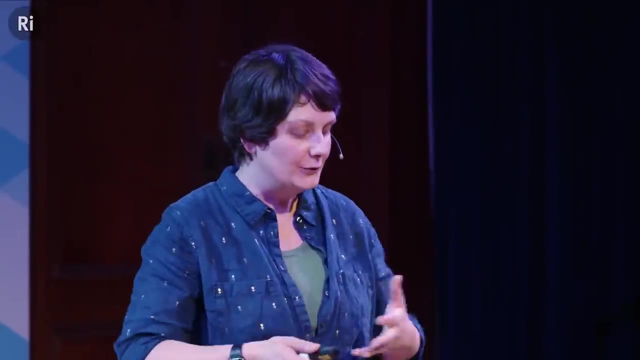 real astrophysicists think I'm a mathematician, But I actually sit in this very interesting and rich space that exists somewhere between the two things. So, especially for Einstein's theory of general relativity for gravity that I'm going to tell you a bit about this evening, it's somewhat 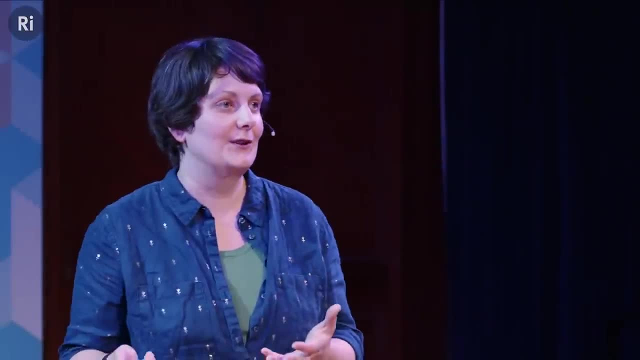 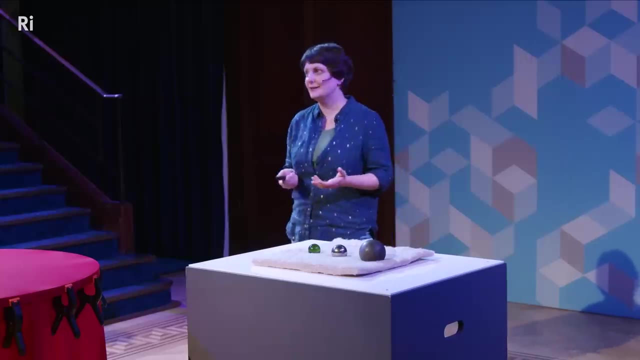 a mathematical theory and yet it has consequences in our universe. So it sits somewhere between the two things. So, as Hassan was saying, this is actually the first in a series of talks that are going to be given by Queen Mary researchers, And when I got the list of all of everyone else's 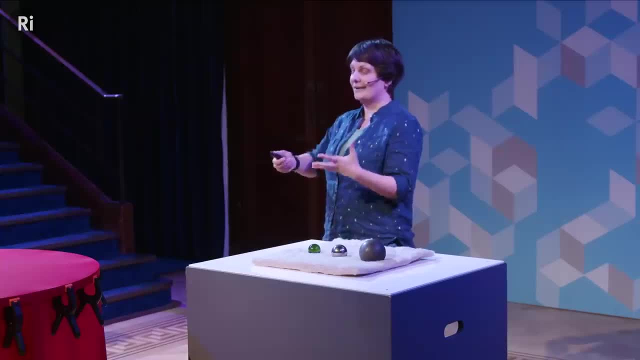 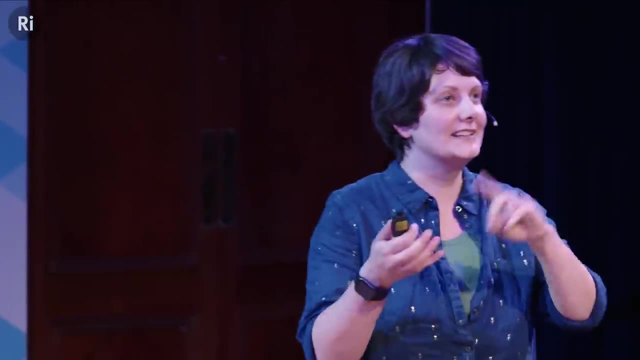 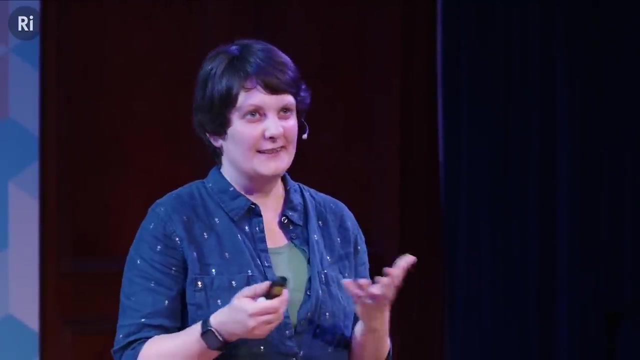 abstracts and titles. I thought, wow, this is really amazing. So there's things like supernovae, exoplanets, beginning of the universe, dark energy, dark matter, all this kind of stuff, And I thought that sounds really impressive. It actually sounds like science fiction. 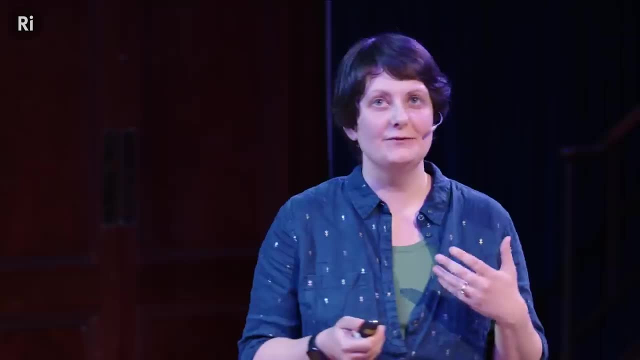 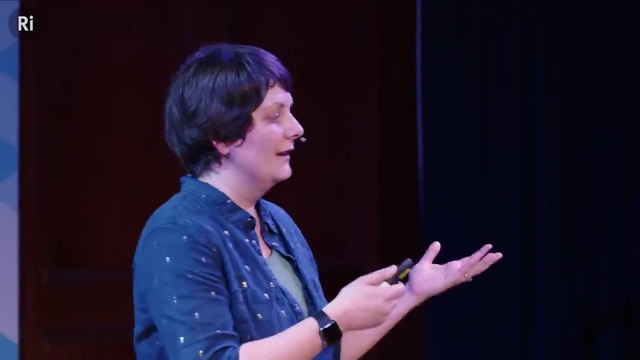 And I thought if I wasn't working in this field, I might find it really difficult to know where the line is between science and science fiction. If I can have all of these crazy supernovae and exoplanets and stuff like that, why can't I have wormholes and warp drives? 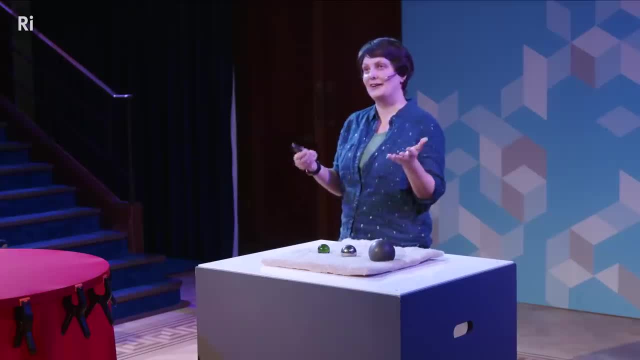 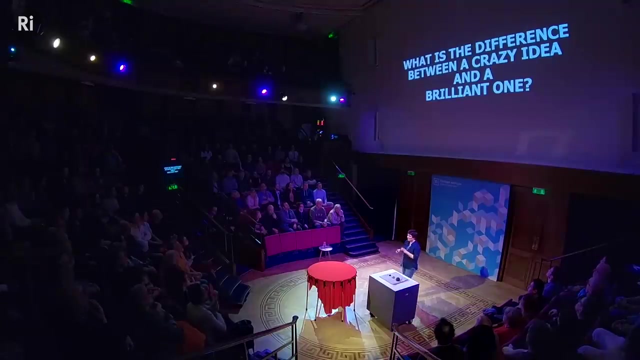 and things like that, And so I thought it would be fun this evening to try and explore with you- which is also, as I say, kind of related to this space that I exist in- for my research somewhere between mathematics and astrophysics. Okay, so let's get started. So an alternative. 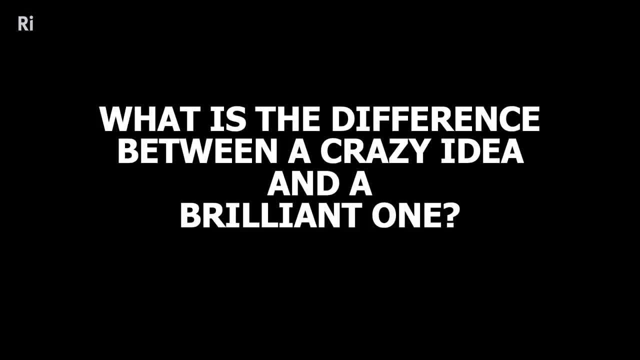 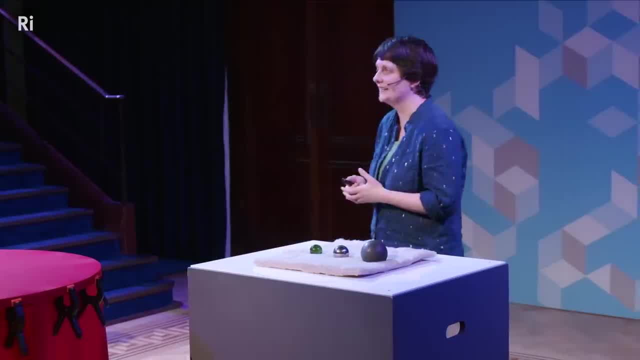 title for my talk is: what's the difference between a crazy idea and a brilliant one? So it turns out, of course you know, if you know anything about the history of science, that we're not very good at telling the difference between these two things. So often we've thought. 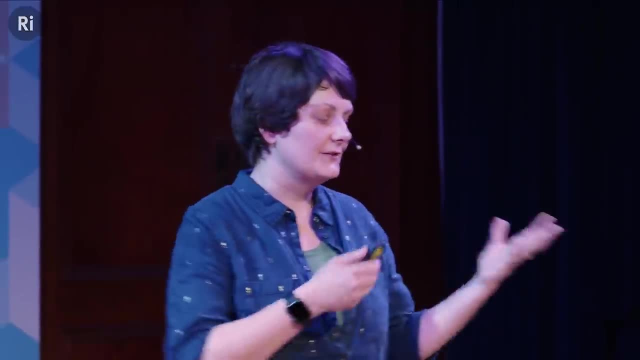 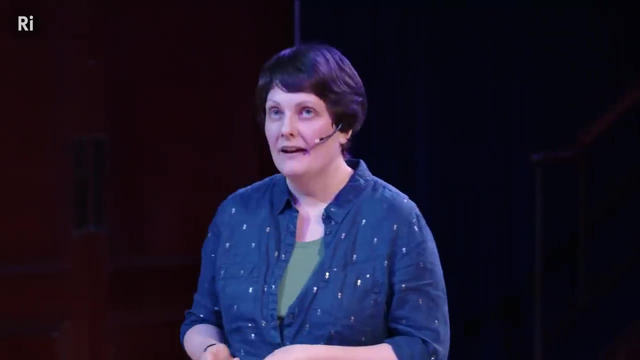 that these ideas and they turn out to be completely wrong, and vice versa. you know things that we thought couldn't be true actually turn out to be reality. you know the reality of the universe that we live in, And so I'm going to focus on three crazy ideas for this evening. 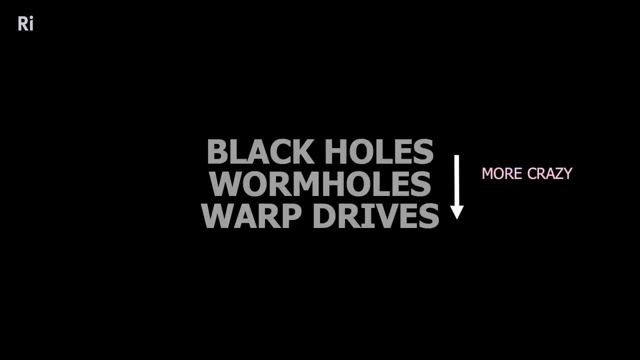 and I've sort of ranked them in order of craziness. So actually, for the second and the third one it's a bit of a matter of taste, Like it depends, you know, how you feel about these things and it depends on the specific type of wormhole. 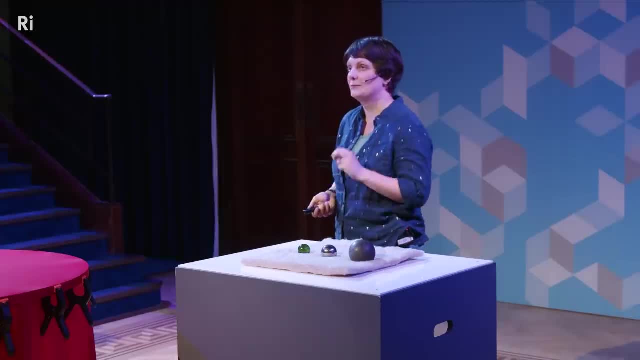 Or warp drive that you want to have, But definitely the first one. black holes do exist. So black holes are really good science and not science fiction, which you know is surprising because they do, as I say, on the face of it, sound kind of completely mad. So before I tell, 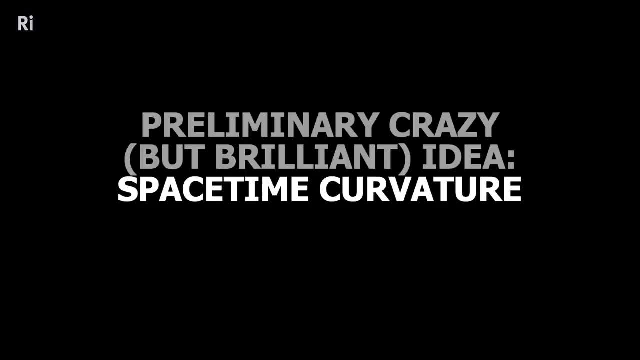 you about these three types of objects. I have to tell you a bit about this really crazy but super brilliant idea, which is space-time curvature. So I think for me, this is one of the most brilliant but also most crazy, and I think it's a really good idea, And so I'm going to. 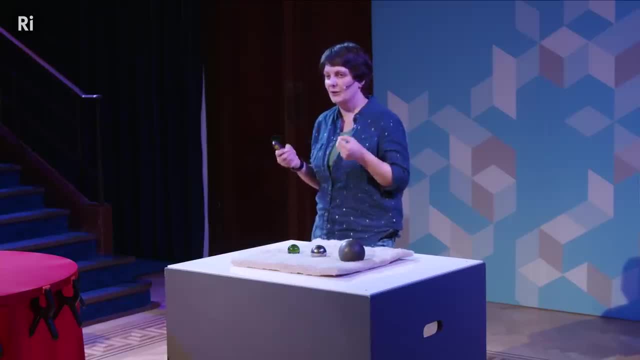 talk about the most crazy ideas in the history of physics. This is one of the things where, when you first encounter it, you just can't accept it. Like deep in you you're like, no, that's not how the universe is, But it is right. It's just that you don't have the right intuition because you 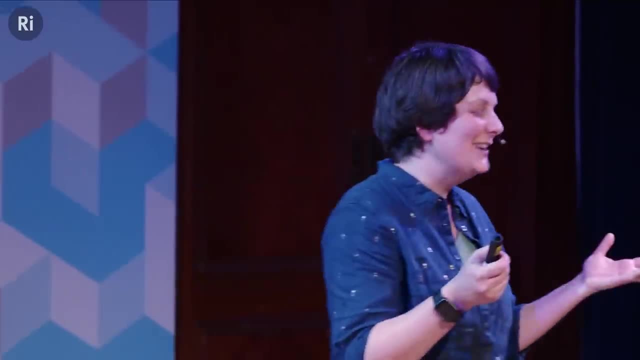 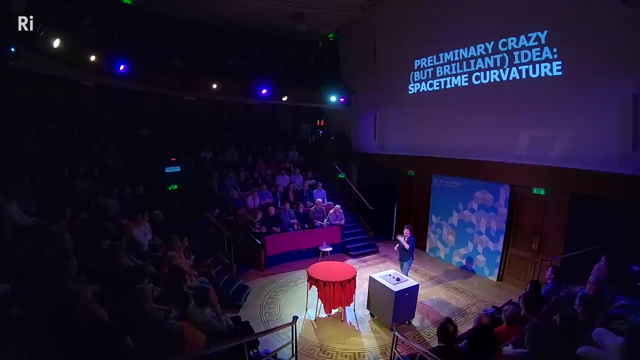 were born and lived most of your life on- well, all of your life, hopefully- on Earth, And you know you've never flown to a black hole or traveled at the speed of light. You know you've, as far as I know, you've all been here for your life. 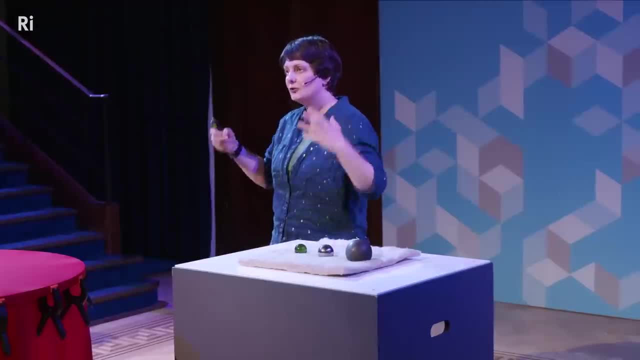 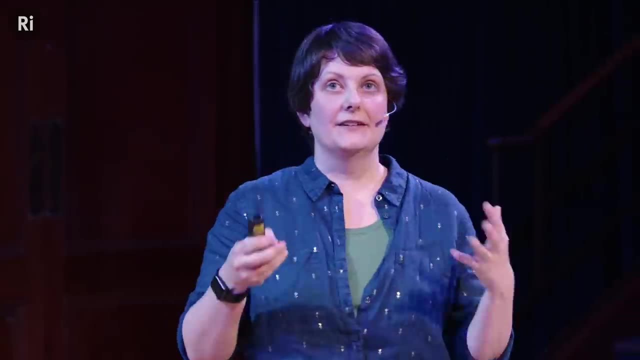 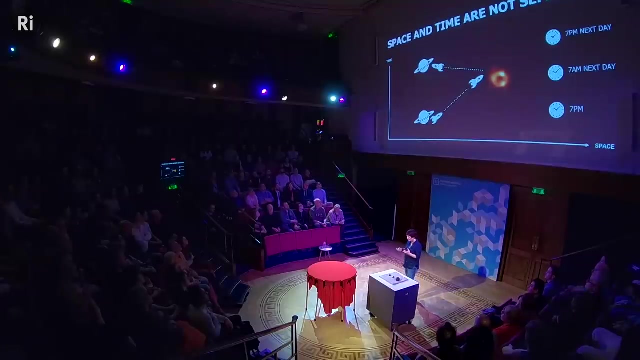 So you just don't have the right intuition for these very strong gravity environments that you have, for example, around black holes. So at the core of this idea is this idea of space-time curvature. So let me break it down for you a bit. So the first part is space-time. So this: 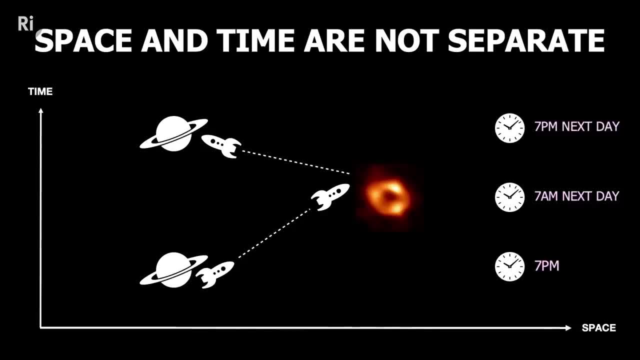 idea of space-time is that somehow, space and time are not separate things, They're not independent. They somehow depend on each other, So they're part of this bigger thing called space-time. So in this picture, this is probably how you normally we would think about space and time. So, along the 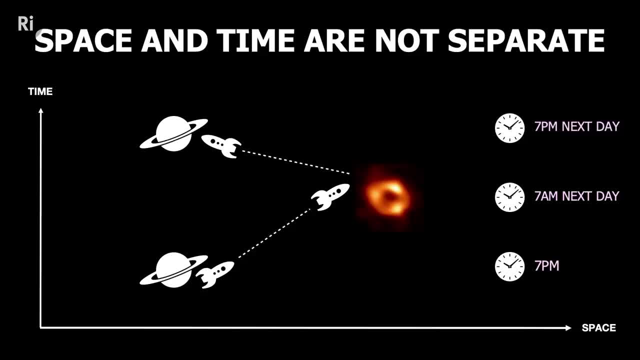 bottom there's space and going upwards, that's moving forward in time, And you would think that you know you flew off from your planet to a nearby black hole or star and you know everyone agrees that you left at 7 o'clock in the evening and you arrived at 7 am the next day, in time for 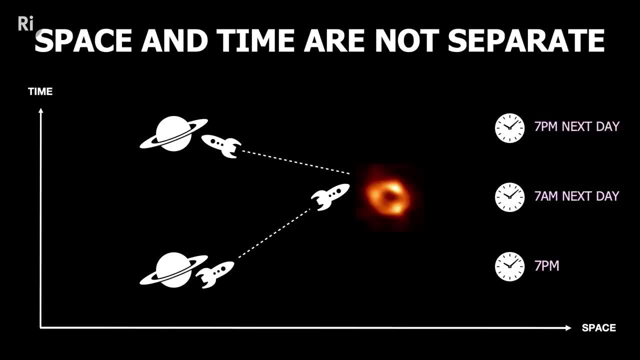 breakfast And then you fly off from your planet to a nearby black hole or star and you know, you turn around and you fly back to your planet And in this picture of time that we have, everyone agrees on the time at which these events happened. right, There's like some big clock in. 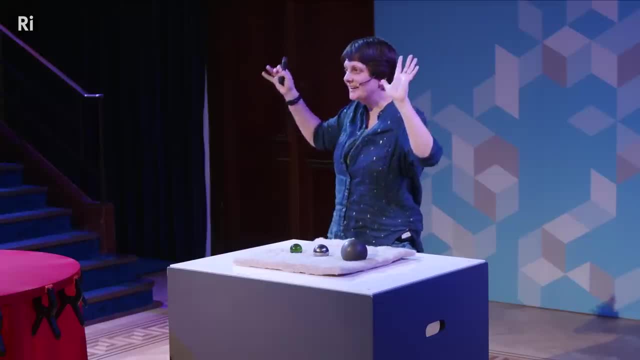 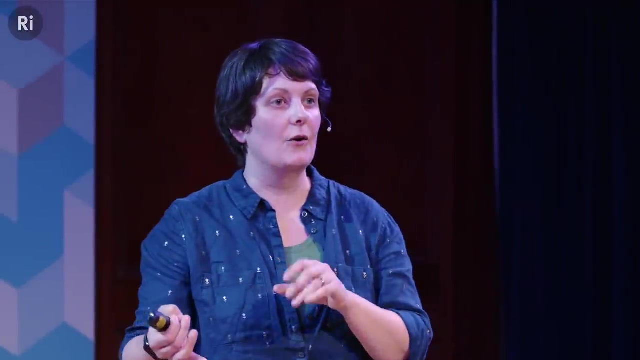 the sky that everyone agrees on, But the reality is there is no such big clock on the sky right To measure the sequence of these events, you need to be the person at each one of them. You need to be the person traveling in the rocket or sitting on the planet or sitting at the black hole, And 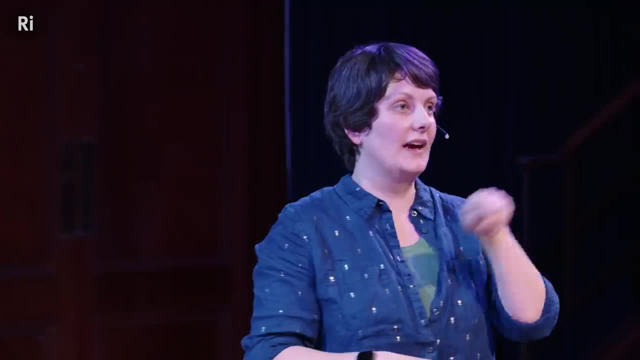 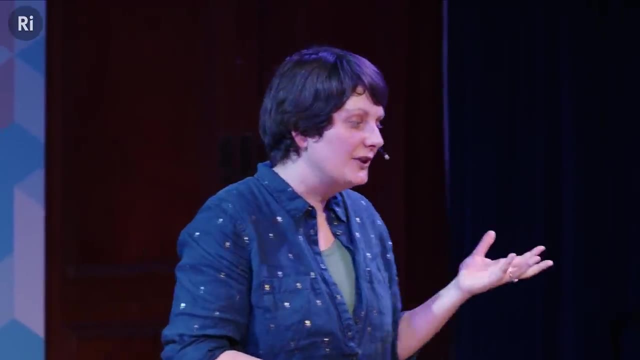 what you see on your watch will differ depending on where you are and which of these events you're at and how you're traveling through the space and the time, And that is, as I say, very counterintuitive, but it is really how our universe works. The second thing that you need to 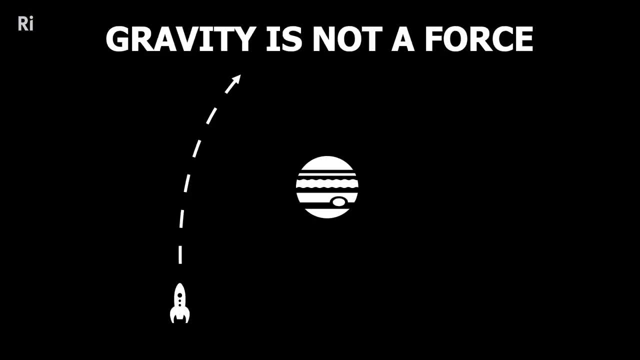 know, and this is again, it's probably deep in you because it's one of the first things you learn when you're at school, Like, I think, really the first science lesson you have. you have to learn forces and you learn magnetism and you learn gravity. So you say: 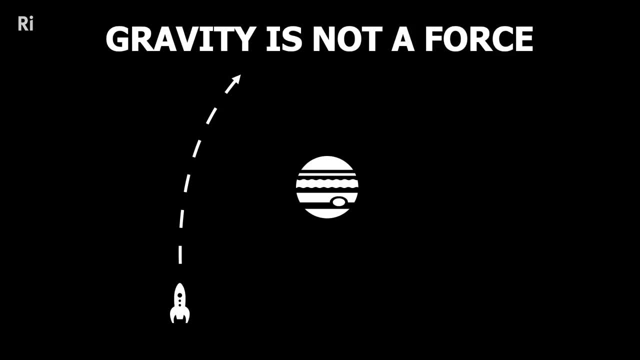 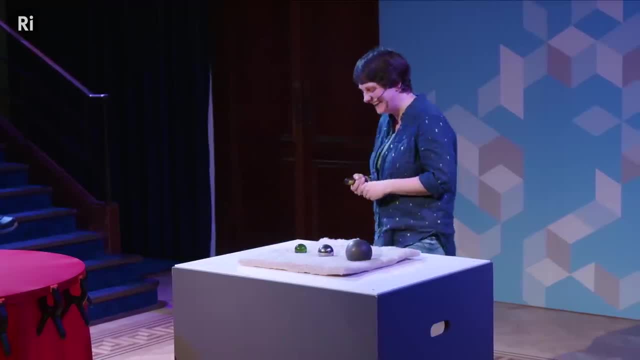 name a force and you say gravity. but that's wrong. okay, We shouldn't actually teach children this. I actually think we should just teach them space-time curvature directly, but I'm apparently a minority view here. So, yeah, we teach them. it's a force which is okay, you know, works on the 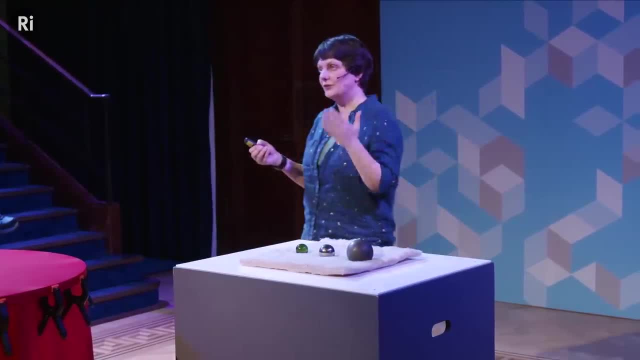 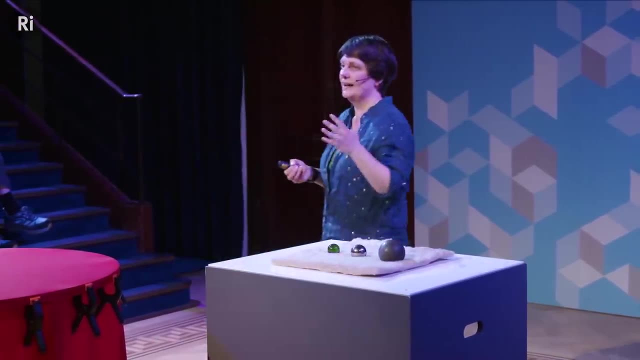 surface of the Earth. So, but you know what is a force. So the idea of a force is that it's something that changes your speed or direction. So in this picture particularly, I'm thinking about a change of direction. So I'm flying my spaceship past a planet. 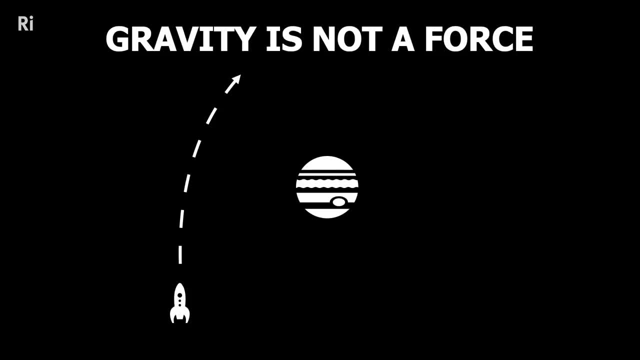 And it gets somehow pulled off course by this gravitational force. And you know we think of this as being, like you know, a kind of like a big magnet that sort of attracts the spaceship towards the Earth. But what I want to tell you is that that's not what's really happening. 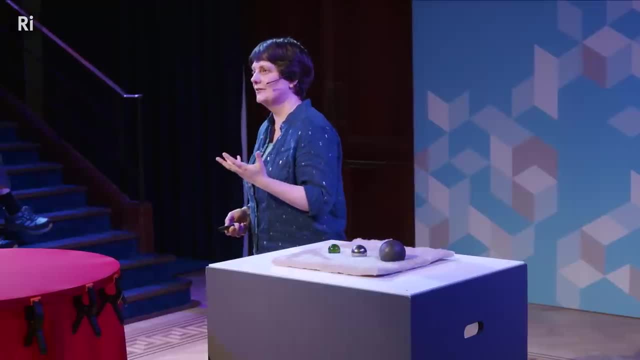 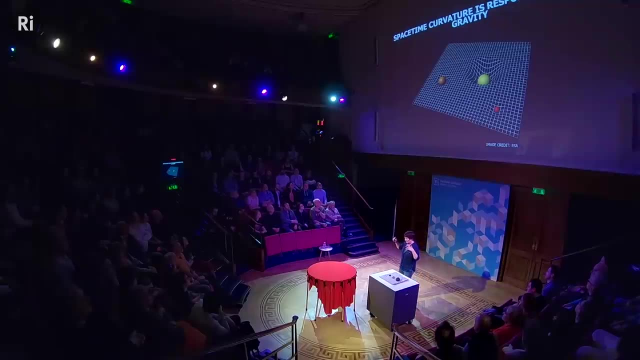 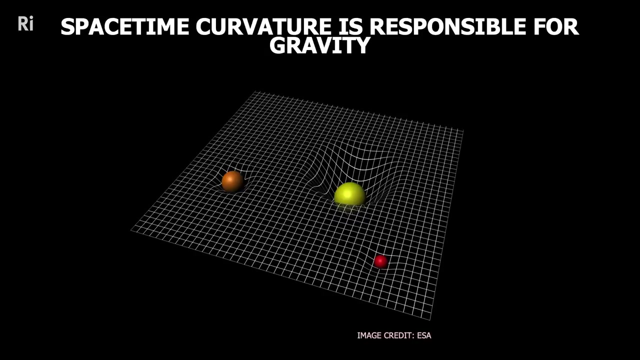 So in fact, we would say actually that there is no change of direction. So the picture that we should have is something like this: that it's not a force that's pulling us off course, it's a curvature, So I have it up on this slide. but Hasan told me you have to do a demo. And I said: 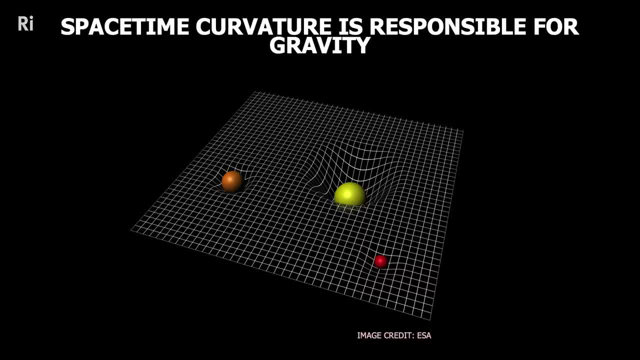 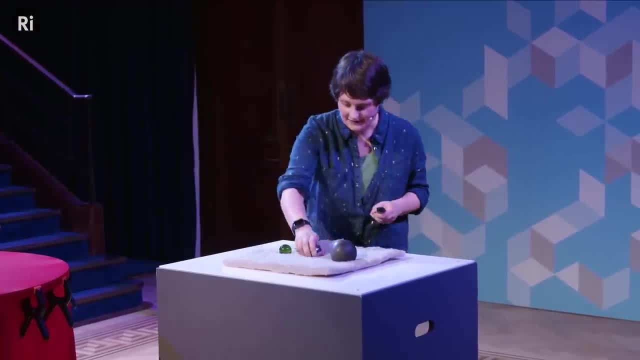 there's a reason why I'm in the mathematics department and not in the engineering department anymore, But okay, so he's responsible for anything that would happen, But okay. so the idea is this. Oh, let me start with a small one. So the idea is basically that you have to imagine: 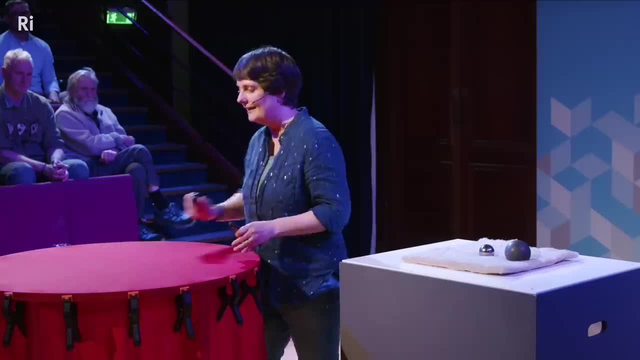 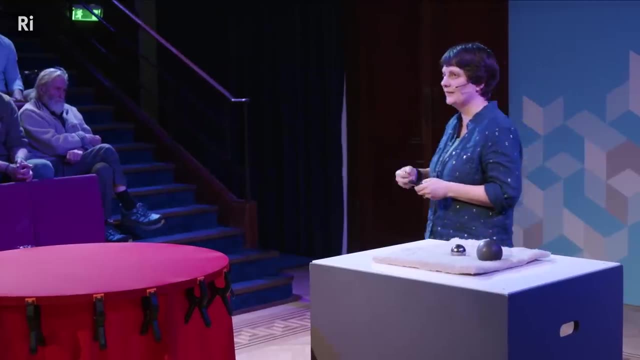 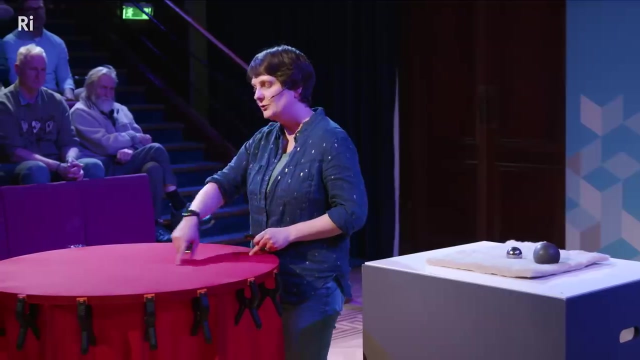 that this two-dimensional surface, this sheet here, is space-time. So that's the first thing that I'm going to do. So people always show this kind of picture when they explain space-time. But this, you know, this sheet has two dimensions. You know it has. I can describe it by two. 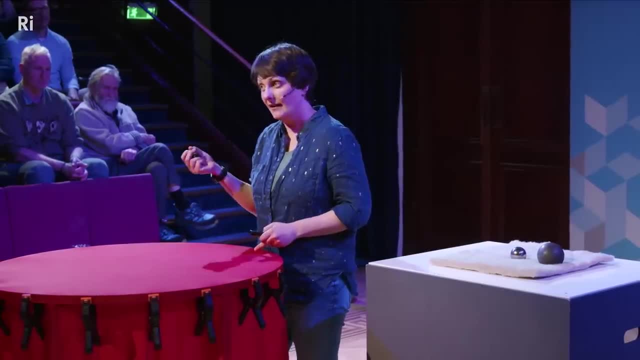 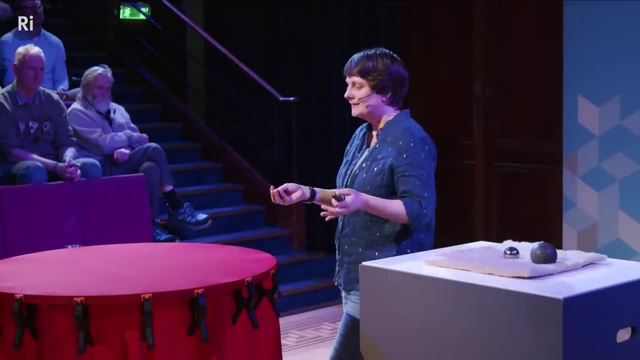 coordinates, But it's supposed to represent space-time, this unified space and time thing that I was talking about, And so it should really be four-dimensional. So already something three-dimensional, you know, like a ball is okay, you can imagine that, But four-dimensional. 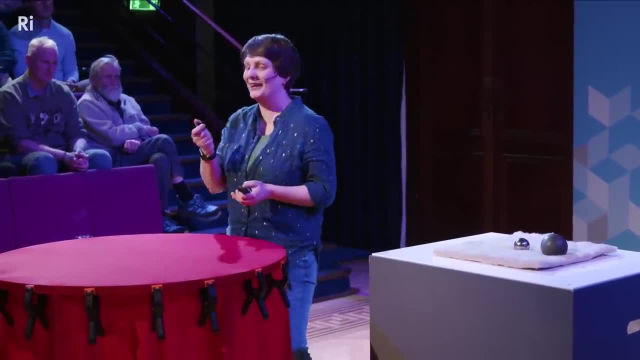 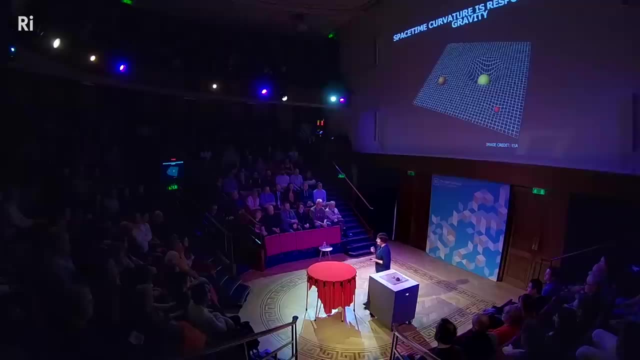 maybe not right, It's. it's okay, right? You don't have to imagine four-dimensional space-time. I actually challenge anyone who says that they can imagine four-dimensional space-time. I don't think they can. But it's okay. As I say, it's just kind of schematic. So just take it as being schematic. 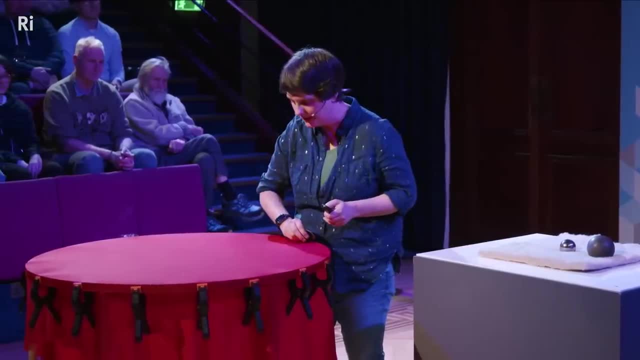 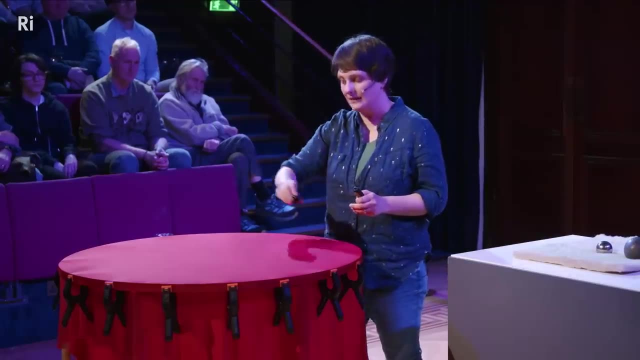 So if I I mean, this is my rocket, this marble, If I roll it across space-time, because it's quite light, it's quite small, it doesn't curve space-time very much, And so it just travels in a straight line. 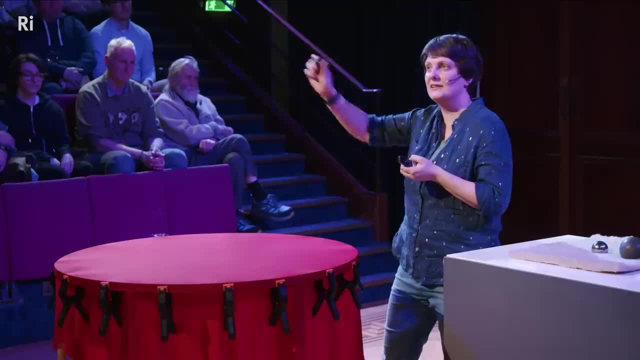 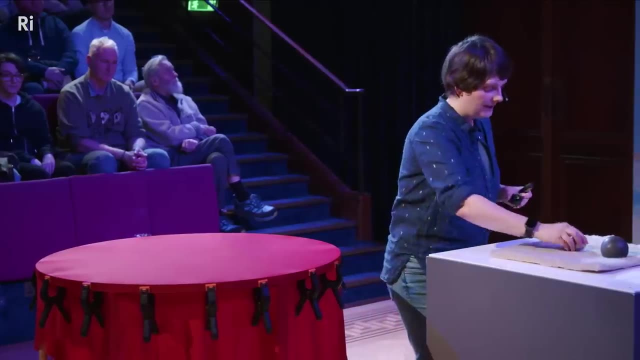 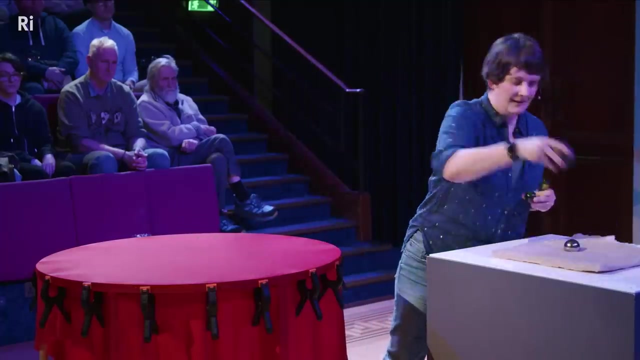 So this is like in a space where I'm travelling through empty space, Right, And I just always move in a straight line. But what if I then put a star in the centre of my space-time? Ooh, That's not enough. I have to do a bigger star. Here's a bigger star. Okay, Now my space-time. 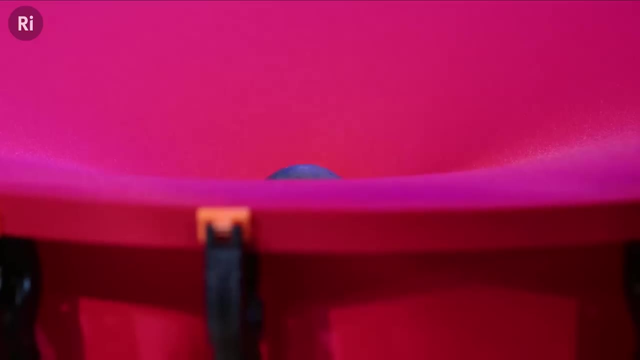 has been curved. So the nice thing about this picture is it tells you where does this, this curvature, this space-time curvature, come from? If you're a big man, you know that's a big question. You should always think: then provide you don't know What is space-time? 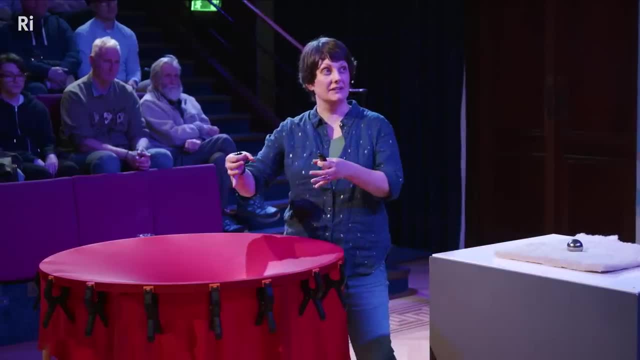 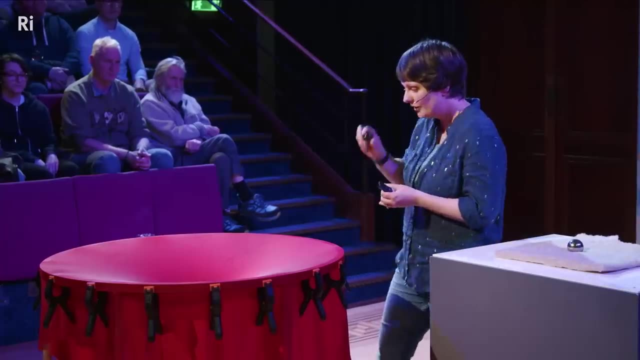 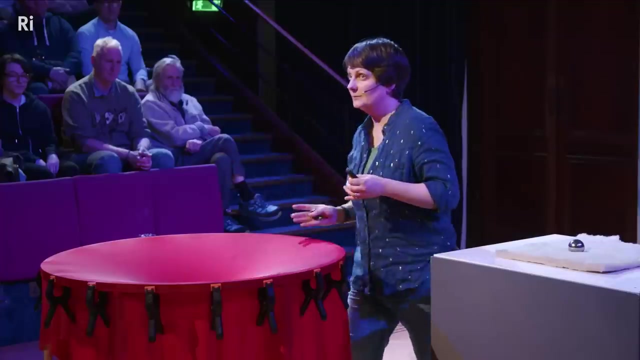 to come from. It comes from energy and matter, So things like stars or planets curve the space time around them, And so then, when I come in with my little rocket, what I can do if I well. so if I try and go in a straight line, I get deflected right, I get pushed off course, And so we might. 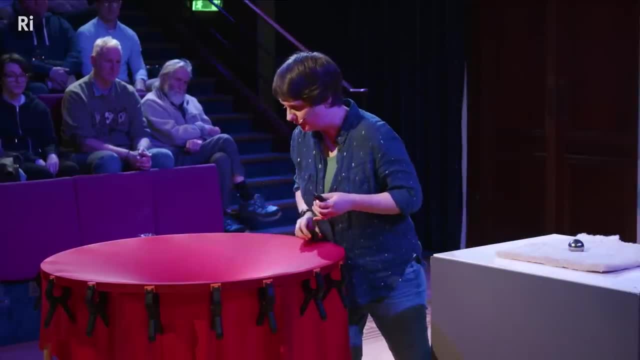 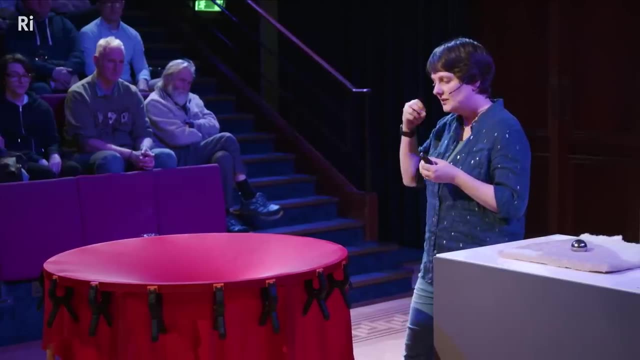 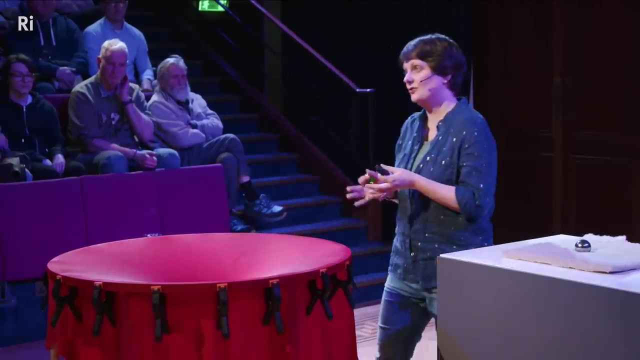 describe this as being a force that's pulling this marble towards the star, But you can see that's not really what's happening, right? So actually, what it's doing is it's following the contours of the surface And because it's a curved surface, those contours are not straight lines. 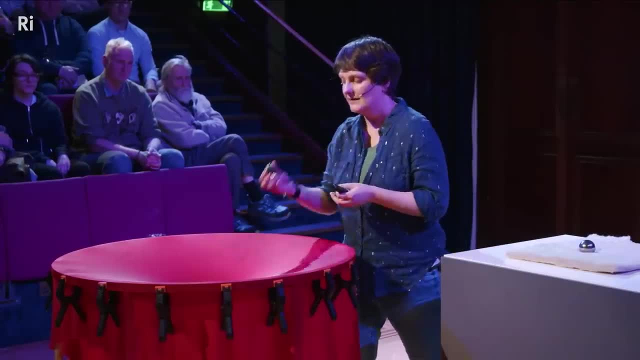 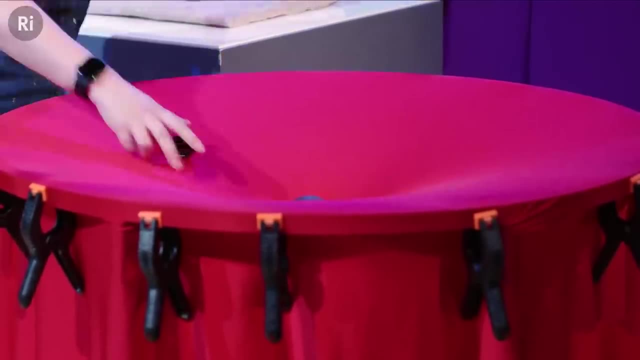 right, They are curved. So there's no magnet in this ball pulling this ball towards it. It's really just following the curvature of my space time. So if I do it- nicely- I'm not very good at this- If I make it do it like this, I can actually get it to go around in an orbit. 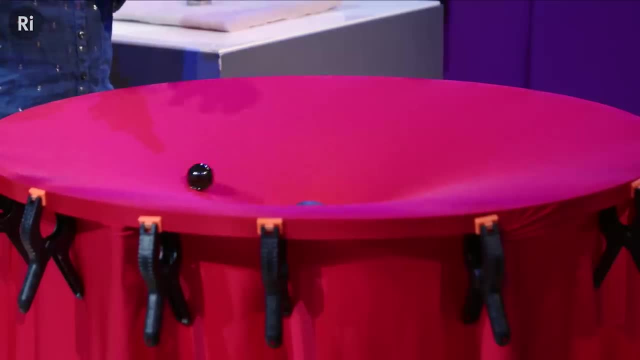 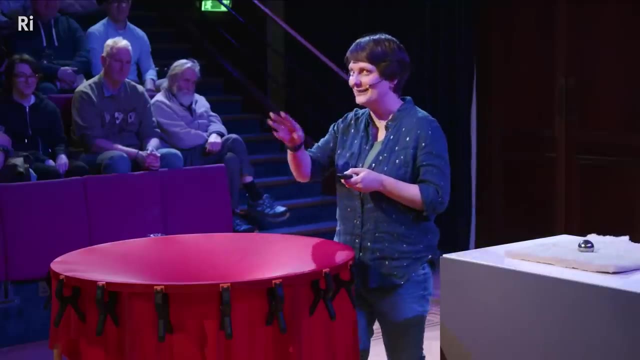 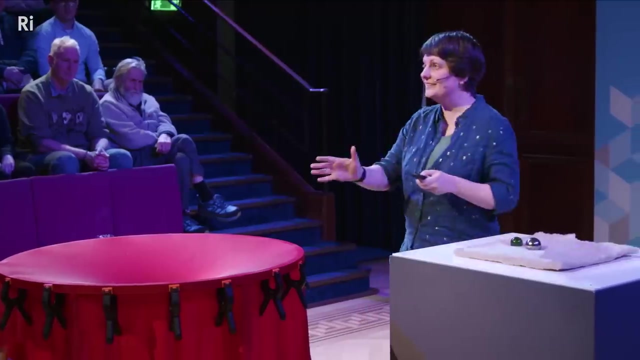 And so this is actually what's happening with the Earth around the sun and the planet around the sun. Okay, We don't in-spiral so fast, don't worry. It takes a very long time for us to in-spiral towards the sun, And so we're all good. But yeah, so this is the concept of space time. 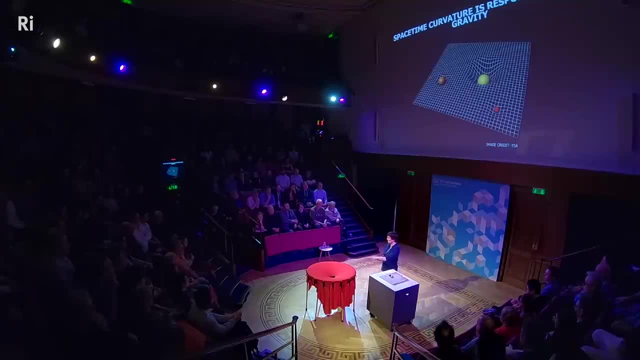 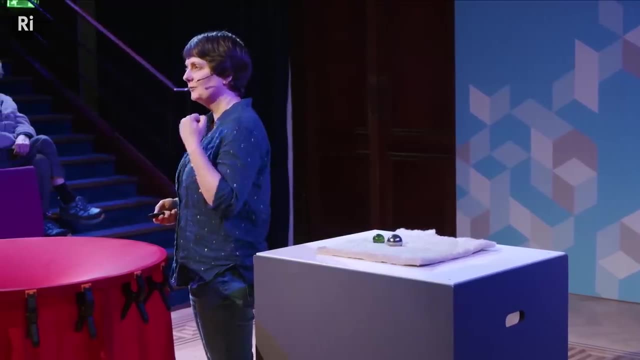 curvature And this is going to be fundamental to all of the objects that I'm talking about. So I'm going to show you lots of these two-dimensional pictures which, you have to remember, are kind of schematic representations of four-dimensional space time. Sorry, I don't need my next two slides, because I did it for you. 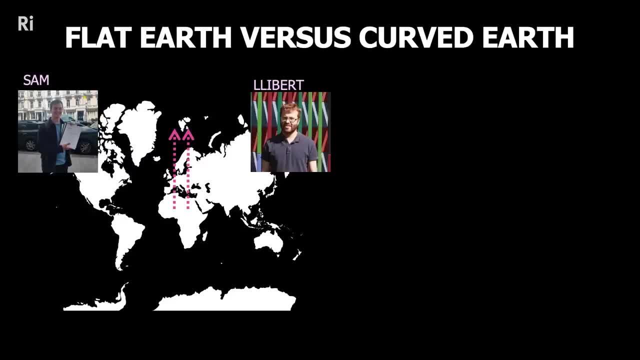 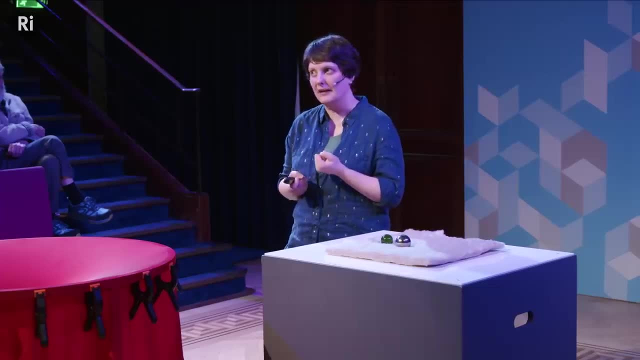 Okay, But I have another picture that I really like to show. This is the one that I really like when I imagine space time, And the reason is that actually, most of the curvature is in the time direction. It's actually not in the space direction. So to quite a good approximation. 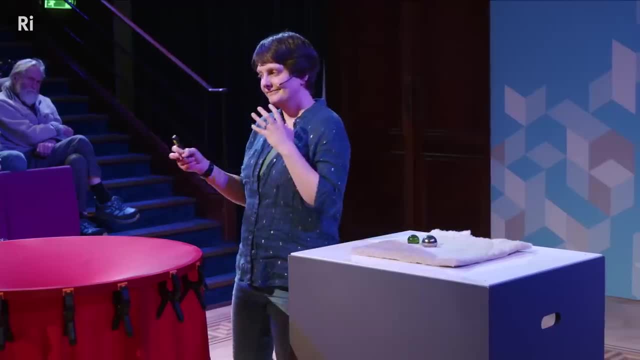 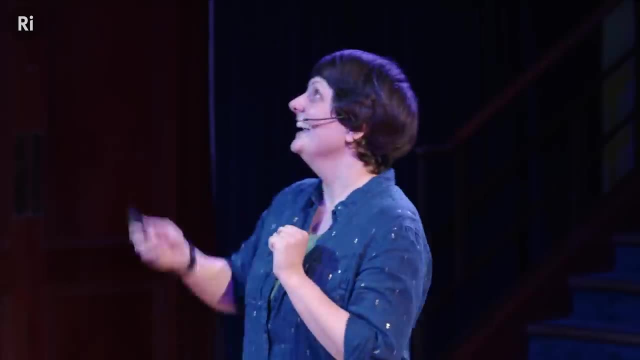 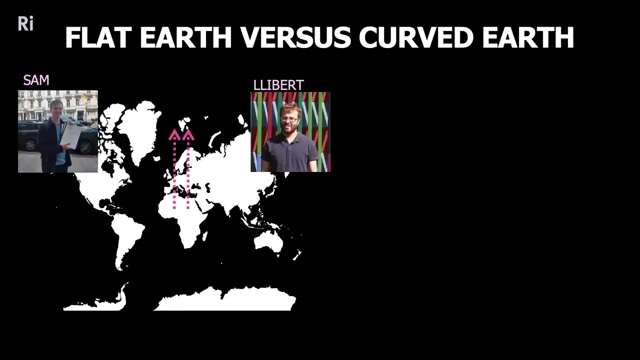 it's time that's curved and not space. Okay, I said they were part of the same thing, So it's a bit subtle, But let me explain with my picture. So here are Sam and Liebert. These are my two PhD students from Queen Mary University. And so I decide: let's pretend that we live a long time. 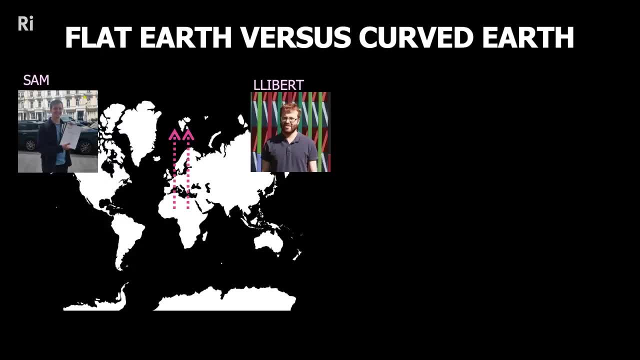 ago. okay, where we don't know if the surface of the earth is flat or curved, And I decide to send my two PhD students to Africa to do an experiment that I can't be bothered to do myself. That's what you do with PhD students. 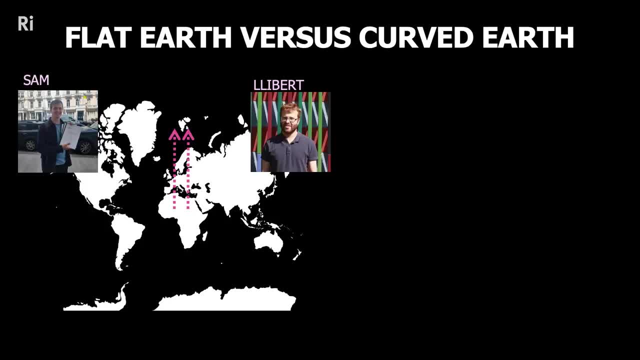 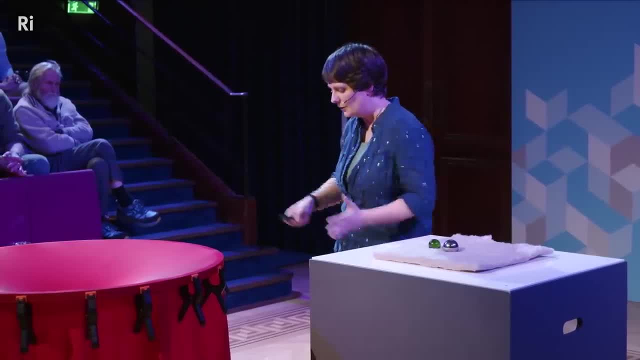 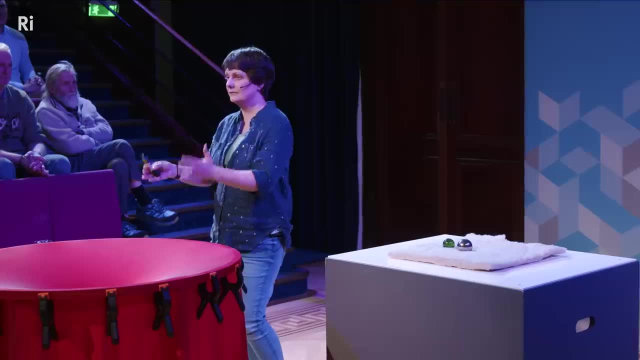 And so I send them to Africa and I tell them: okay, we're going to do an experiment, You need to start at the equator and you're going to line yourselves up, So you're going parallel, right. So one here, one here. And I tell them: you're going to walk in a straight line, right, You're going. 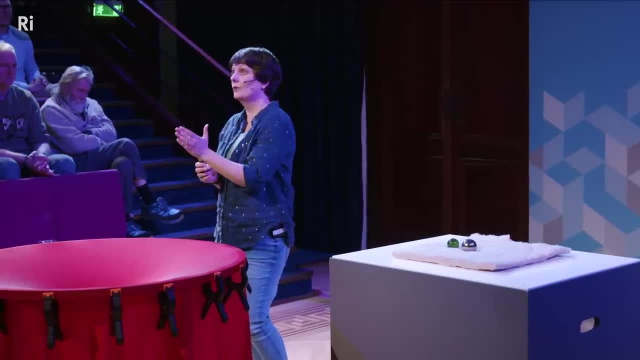 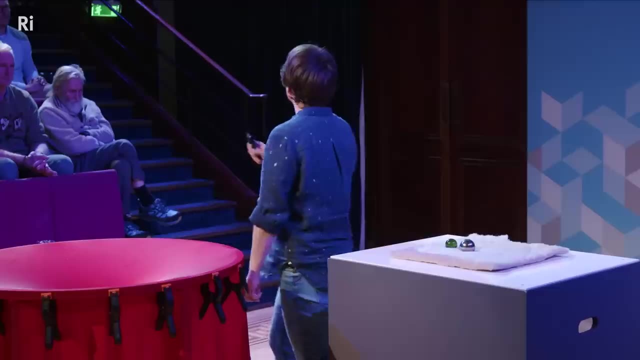 to just fix your eyes on the horizon and you're going to head north. right, You're just going to walk always in a straight line. It doesn't matter if you're being chased by lions, You have to walk in a straight line. Okay, So off they go. 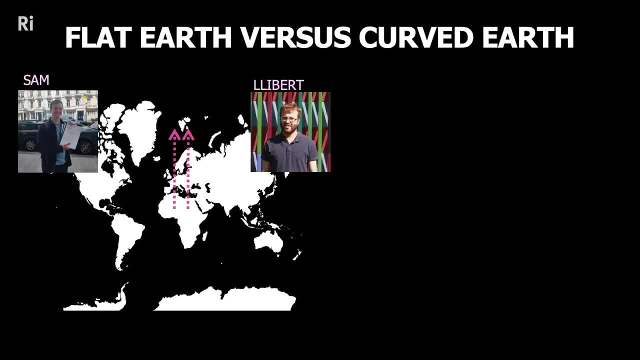 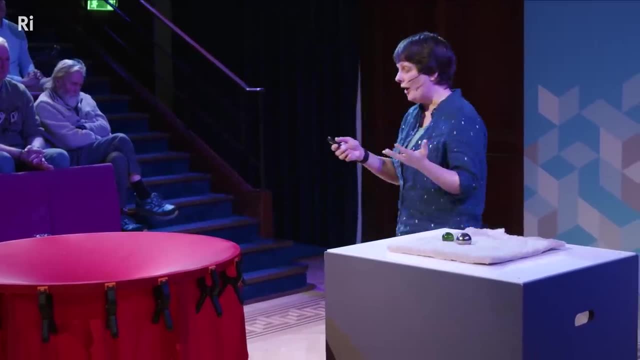 And if the earth was really flat, then this picture is what would happen, right, They would stay separated. They would stay a certain distance apart as they traveled north And when they got to Europe, they would find that they were still the same distance apart. But of course, you know, I hope. 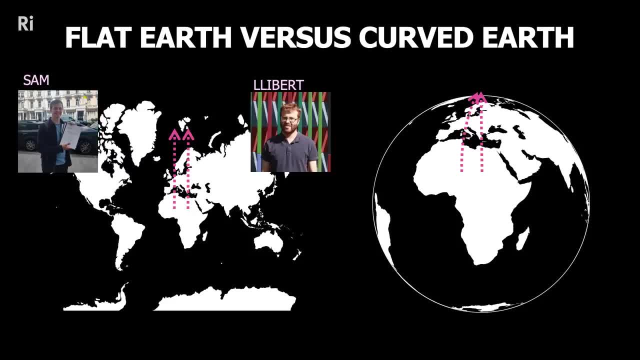 you know that our earth is in fact a ball, And therefore that's not what would happen If they both kept going north. eventually they would find that they were getting closer together. They would actually meet there, right. They would find that they'd been pulled. they got together at the north. 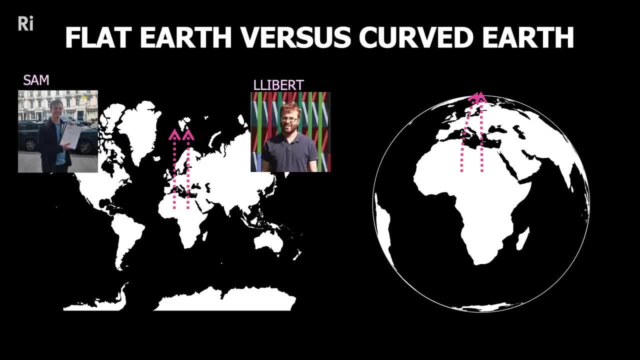 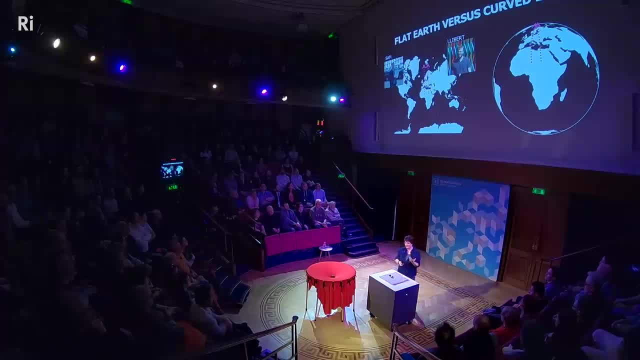 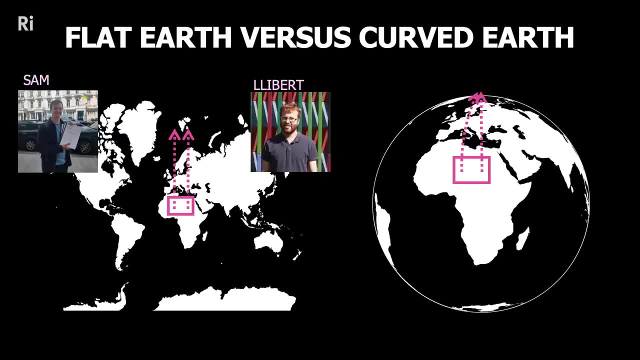 pole, And so they might sort of be kind of confused about that if they thought that the earth was really flat. So the reason that we thought for a long time in the history of people that these pictures were the same is because we live on this very tiny patch of the planet right, So in a very 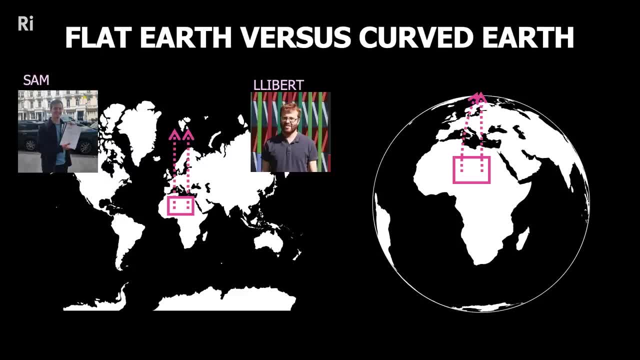 small box. these two pictures look the same. People stay the same distance apart. It's only when you start to travel on distances that are similar to this curvature scale of the surface of the earth that you start to see differences that tell you that it's a curved. 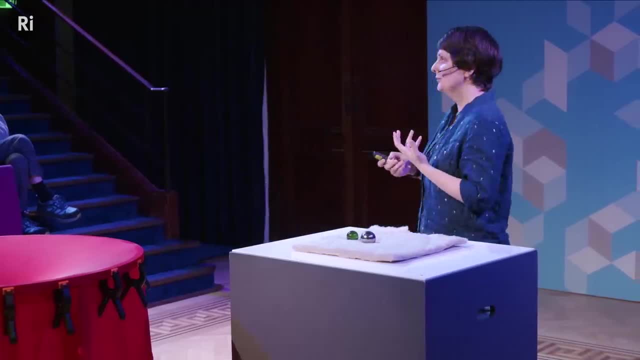 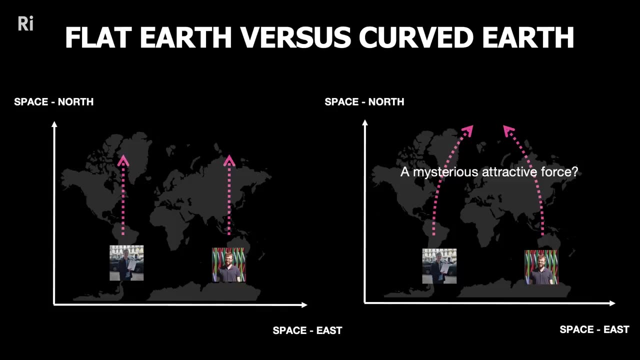 surface. So okay, here's a more schematic picture of what I just told you. You've got north in space and Sam and Liebert are going north, And in the left-hand picture this is flat earth, And in the right-hand picture is what would happen on the actual curve, And in the left-hand picture this is. 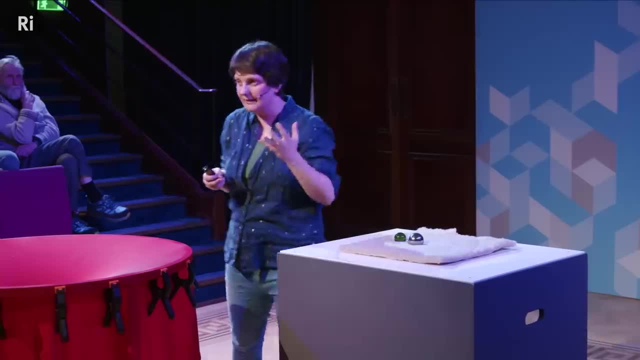 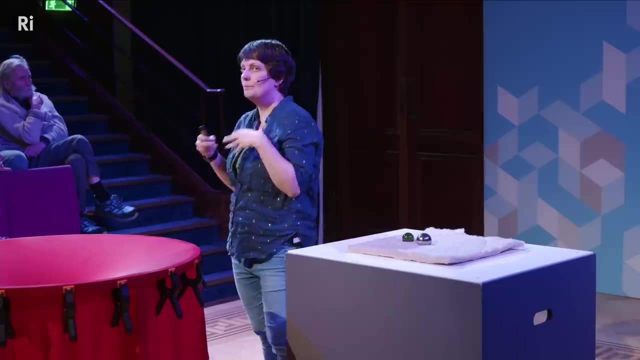 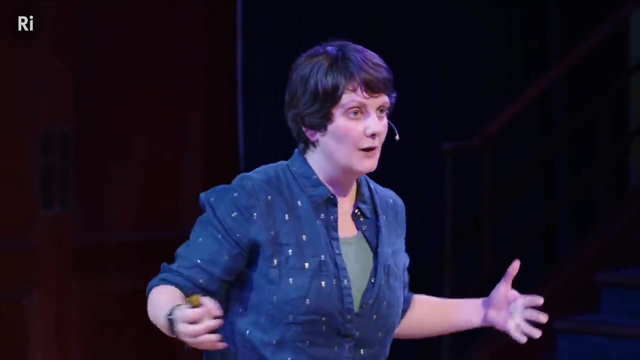 curved earth. But if they were really determined, you know, to hang on to this picture of a flat earth, what they might say is: well, maybe there was some kind of mysterious force that pulled us off course. So we didn't go in a straight line, We got somehow pulled off course, And that's why. 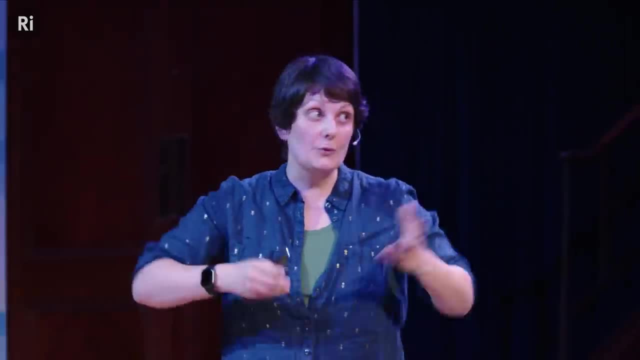 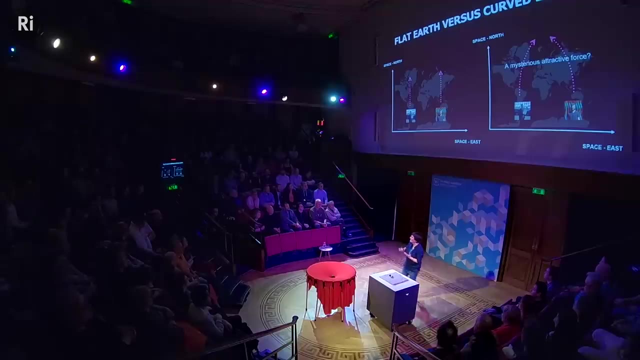 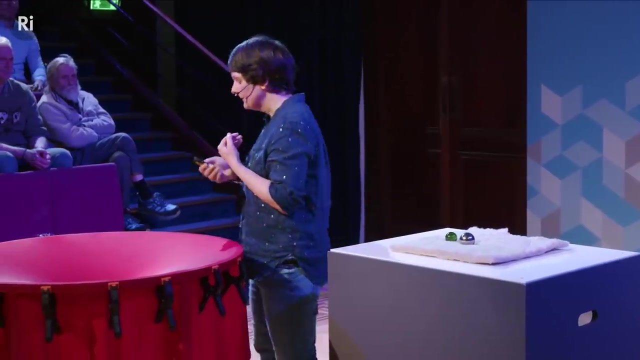 we met at the north pole, So that would be wrong, but they could. you know, PhD students, what can you do? You know, they might reasonably conclude that And in fact they could probably build a model where these two things look the same. So what I'm sort of getting at indirectly eventually, is that this is: 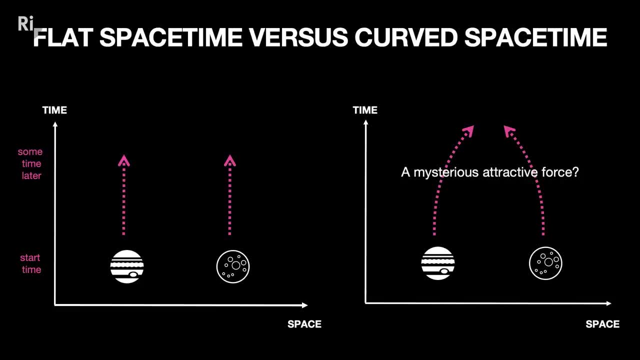 exactly what's happening with space-time and gravity. So this mysterious attractive force. we call that gravity, but actually it's the fact that we're moving now through time and time is curved. So instead of having going north, I've replaced it with time, And so this is exactly what's happening. 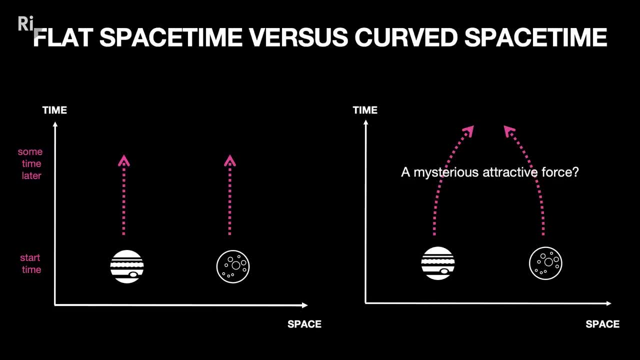 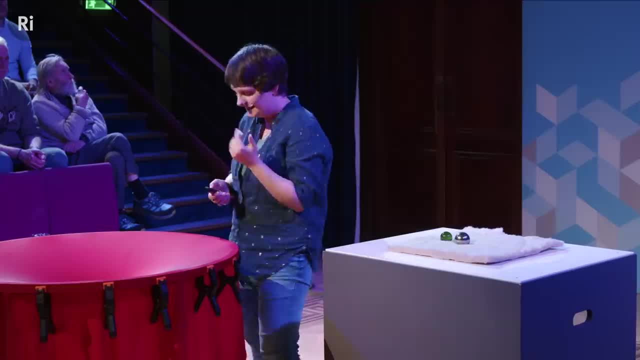 here I've replaced this north axis with time. So that's as I say, that's quite a hard concept to think of time being curved, But that is indeed what happens. And so you might ask me at this point, you know, 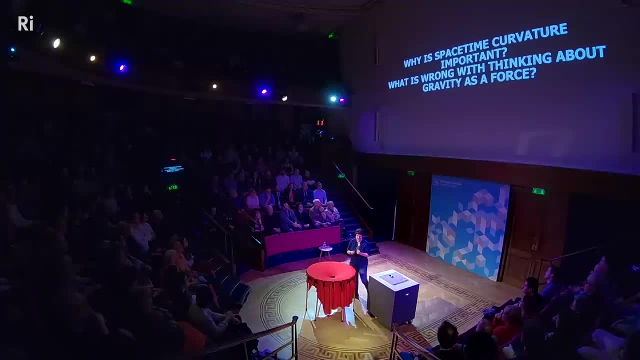 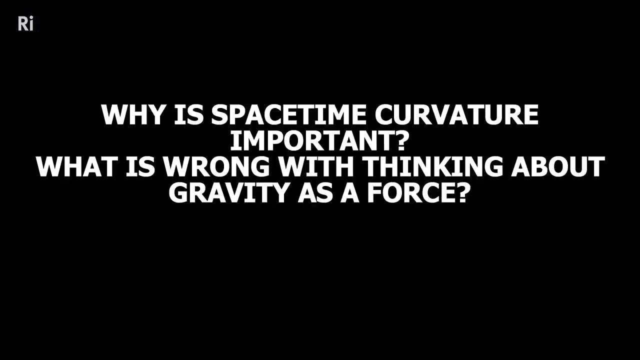 okay, Katie, this is all very interesting, space-time curvature. But to be honest, I've got to this point in my life and I've never needed the concept of space-time curvature. Like just thinking of gravity as a force has worked okay And you know, from a space-time perspective, I've never needed. 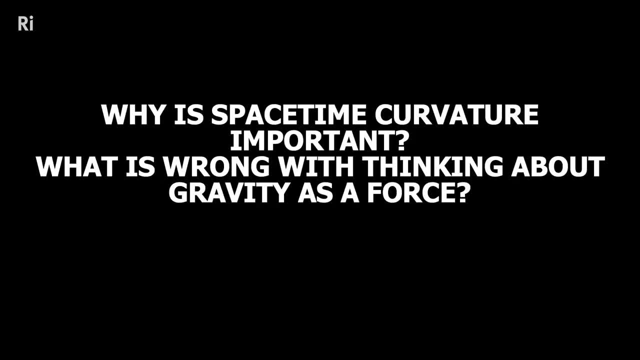 the concept of gravity as a force. But, to be honest, I've never needed the concept of space-time curvature. Like, frankly, what's wrong with just thinking of it as a force if in fact they're just equivalent? But the 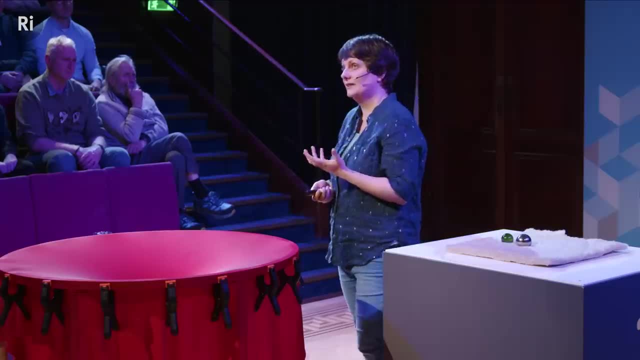 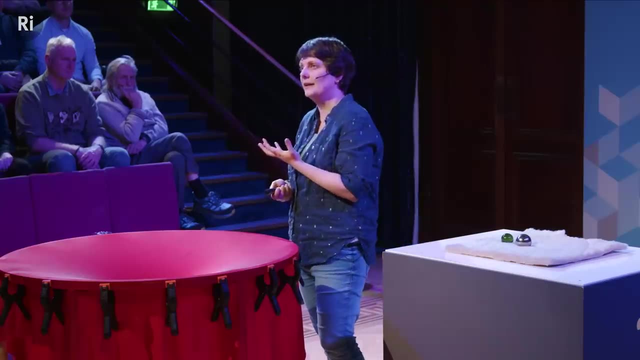 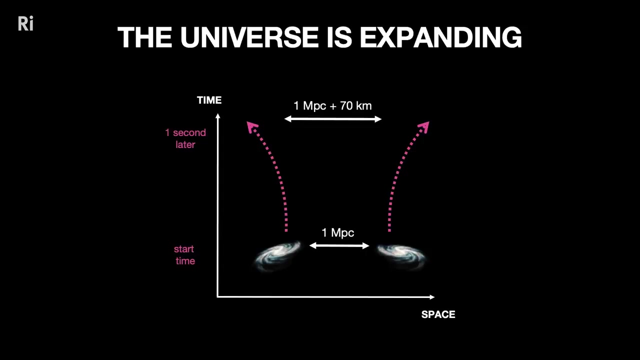 problem is that in some situations they're not equivalent, In some situations they're different And, in particular, in some situations you just can't describe what you're seeing, with gravity being a force. So a really good example of this is that the universe is expanding, And so this is. 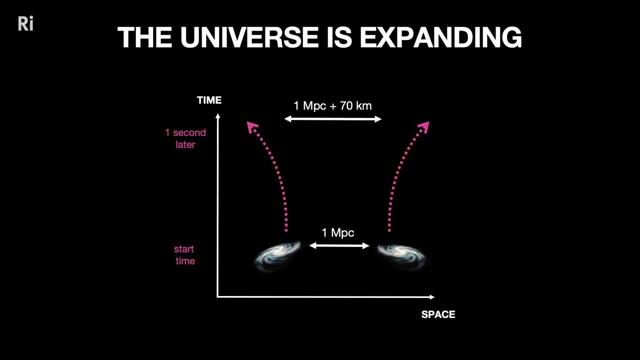 called the Hubble expansion. Perhaps you've heard of it, But what happens is that the universe is expanding And what happens is that if you take two galaxies, so these two galaxies are something like a megaparsec apart. So maybe you don't know a megaparsec, but it's a really long distance. 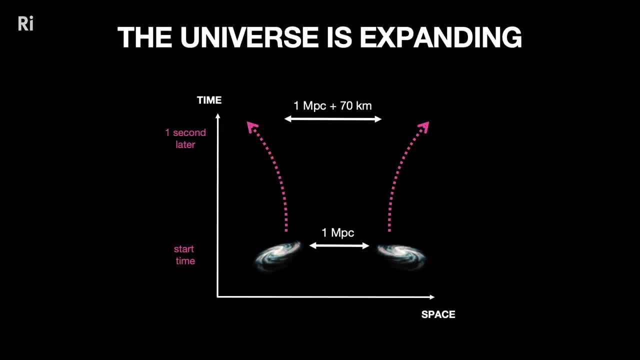 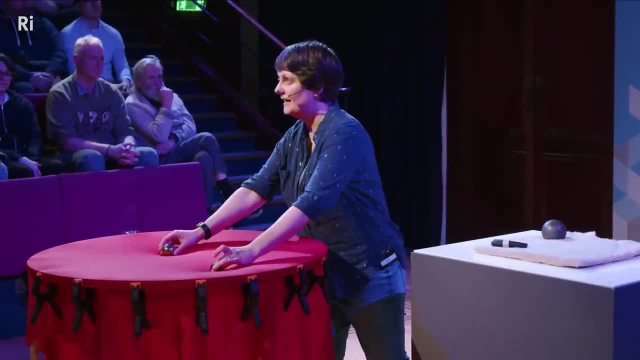 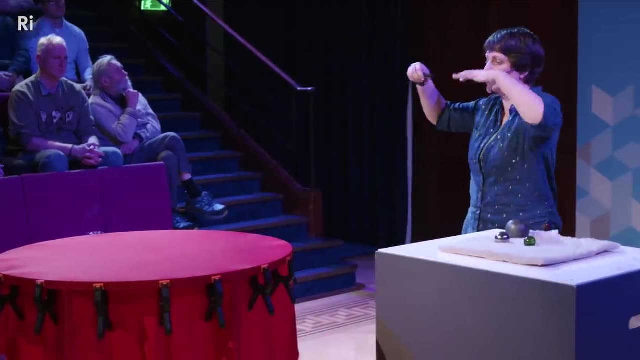 So this is such a long distance that they're individual curvatures. So, if I come back to here, So the fact that they're individually curving the space they're not affecting each other, So they're not being pulled together anymore by this sort of what we would call the gravity of the universe. It's not an gravitational attraction- the force- But it's really down to the curvature around each of these galaxies. So they're really very far apart. And what you'd find if you looked at these galaxies is if they started a megaparsec apart, one second later they would be one megaparsec. 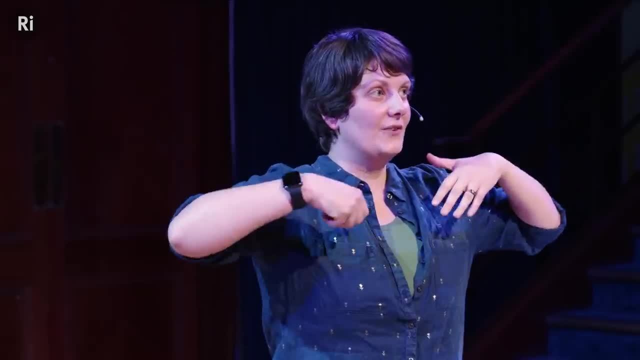 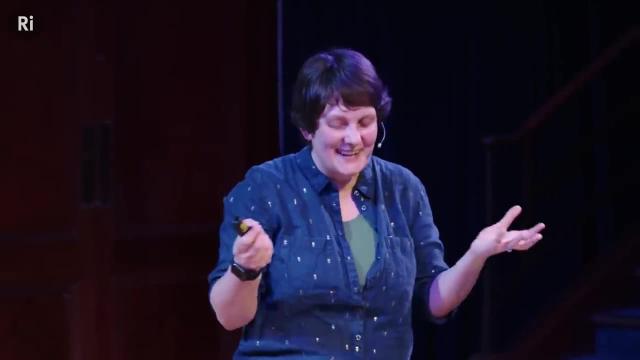 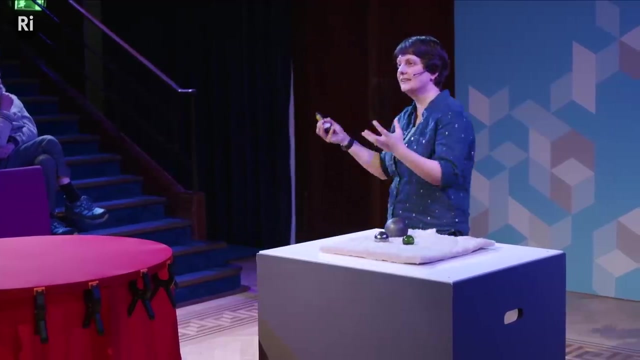 plus 70 kilometers apart, So they're actually moving away from each other. So that's really weird. actually, It's really hard to explain. Like, how do you explain that? How do you explain that Using a gravitational force? These objects are normal galaxies. They have positive mass and 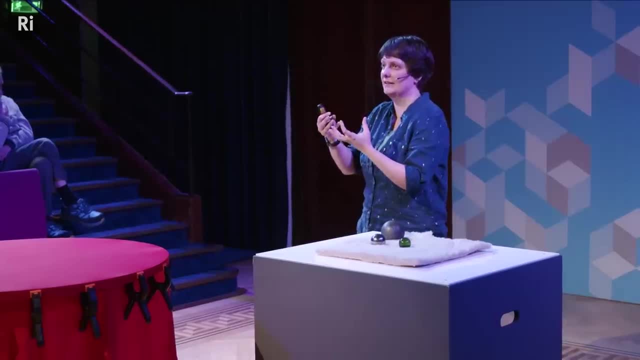 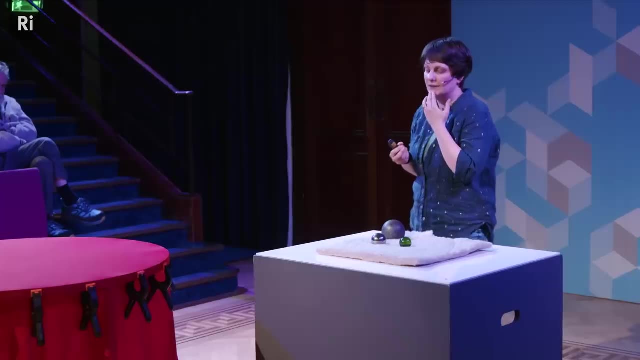 matter in them, And so they should, if anything, attract each other. Or, you know, if they're so far apart, they should just kind of stay where they are. They should just, you know, stay a certain distance apart in time. But what Hubble showed is that in fact, they are moving apart. 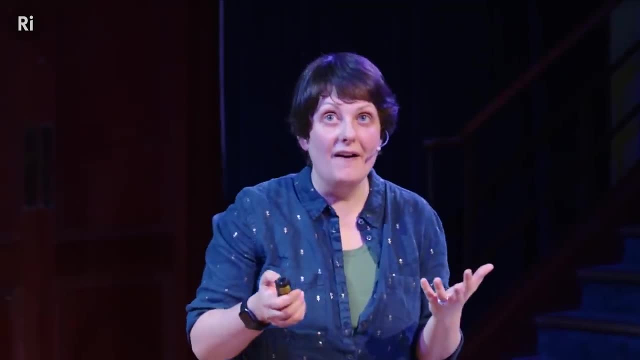 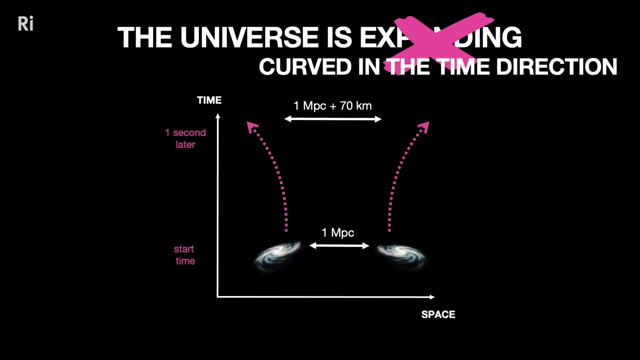 in this way. And the reason that they're moving apart is because the universe is curved in the time direction, And so they're moving apart in this way, And so they're moving apart in this way. So we never say this. We always say: the universe is expanding. I would like people to say the 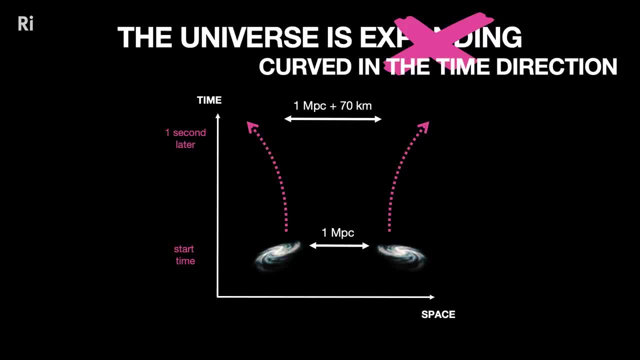 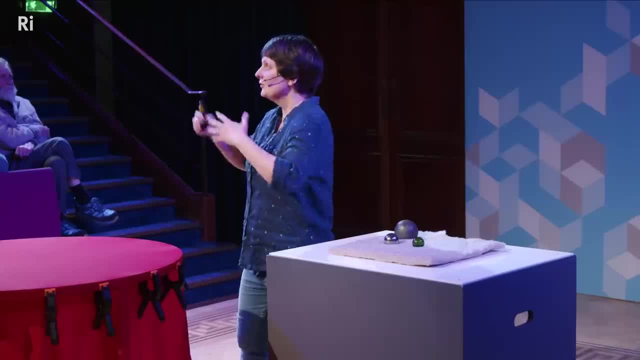 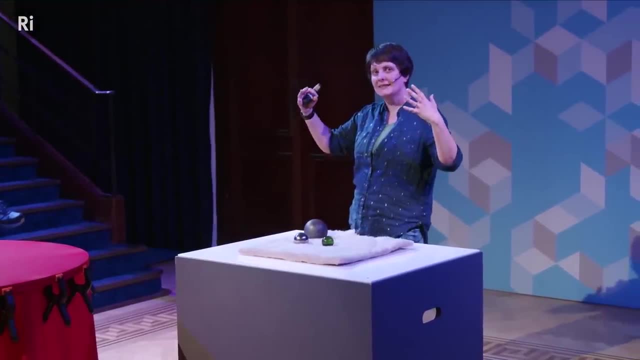 universe is curved in the time direction, but it's not really caught on. So the point is that if you see it in this way, suddenly things make a bit more sense. So the interesting thing which you'll notice immediately is somehow the universe as a whole is curved in the opposite way to how it's. 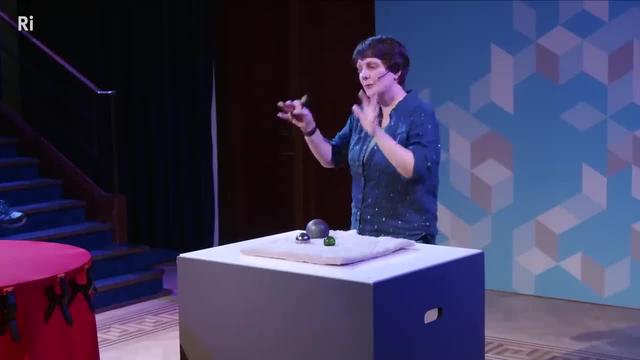 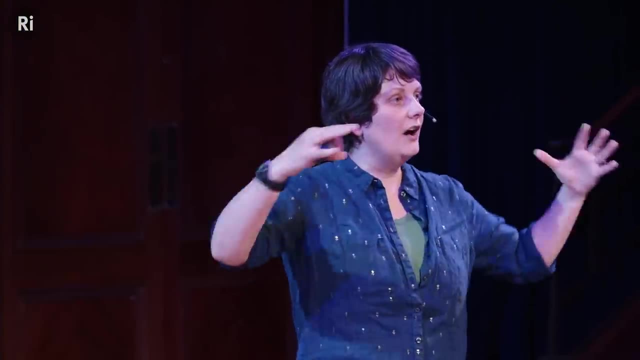 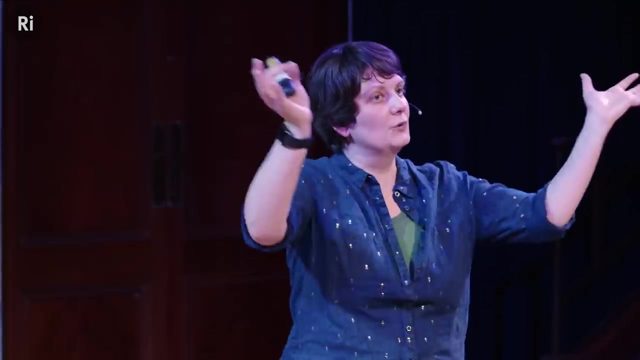 curved kind of locally around objects. So this is completely consistent with Einstein's theory. It can happen this way, But the universe is somehow curved such that, you know, it's like it being curved up instead of down, So instead of things sort of moving together, they move apart. 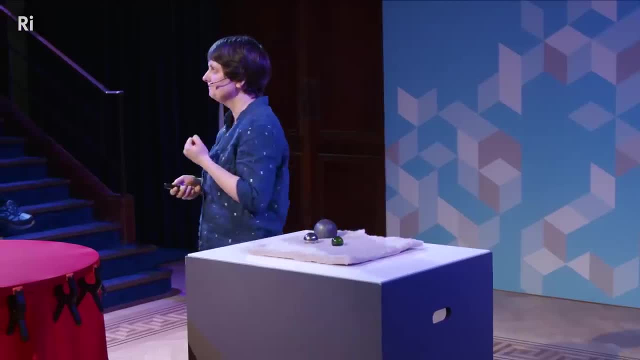 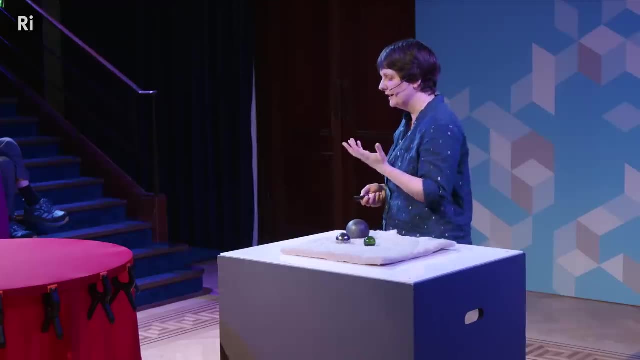 over time, But it's still curvature in the time direction. But, as I say, if you think of it in this way, it's really nice, Because a lot of the questions that people often have about cosmology and about the universe, you start to think of them in what I think is kind of more the right way. You. 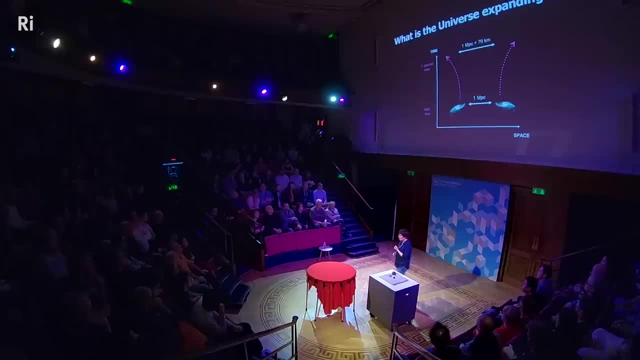 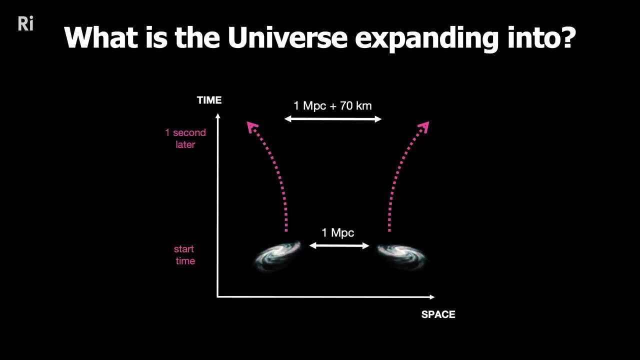 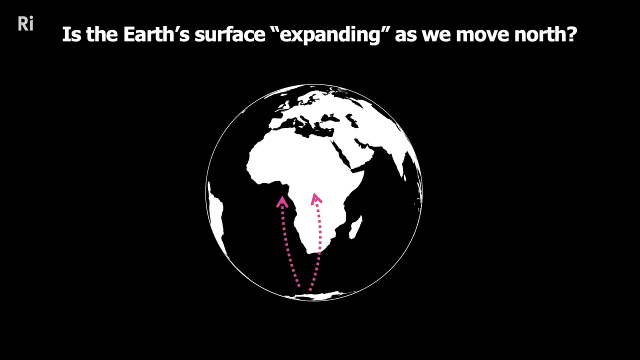 start to ask the right kind of questions. So, for example, one question that people always ask is: what is the universe expanding into? You know, if the universe is expanding, what is it expanding into? But this is like asking what's the Earth's surface expanding into? Or, you know, would you describe? 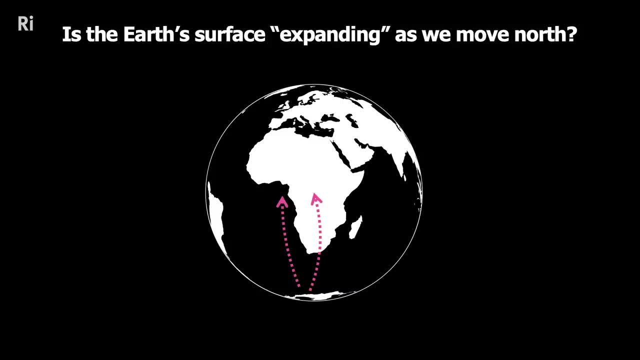 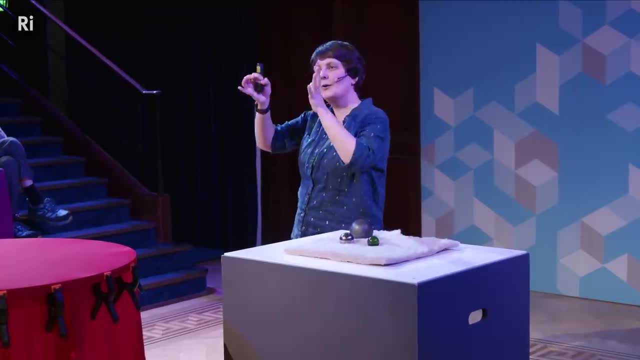 the Earth's surface as somehow expanding as you move north. I mean, you kind of could describe it in this way: You know, somehow the Earth kind of gets bigger. You know you kind of get bigger, You know, as you get north, But it's not really expanding, It's like it's. you know it's already there And 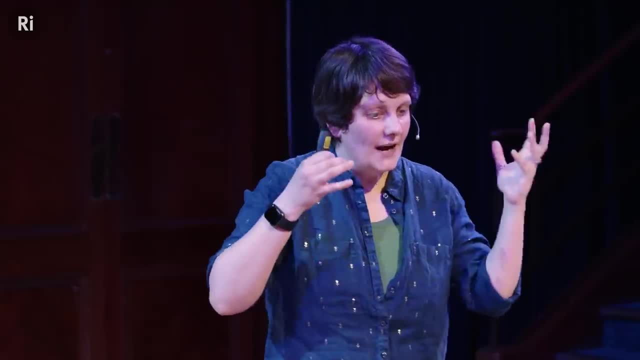 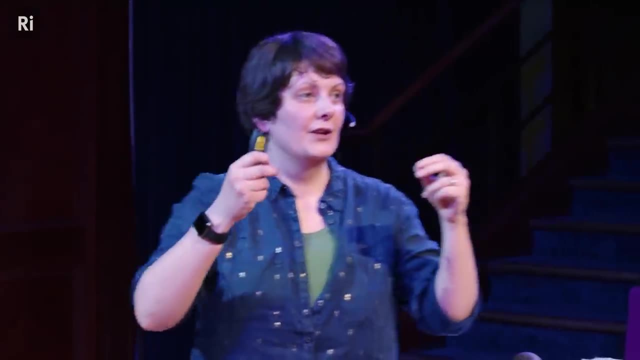 we're just moving on this curved surface. So this is, in a way, how you should think about our universe, that it's just this kind of curved surface. So a more interesting question is to ask something about: you know, can I go round the universe right Like I can go round the Earth? 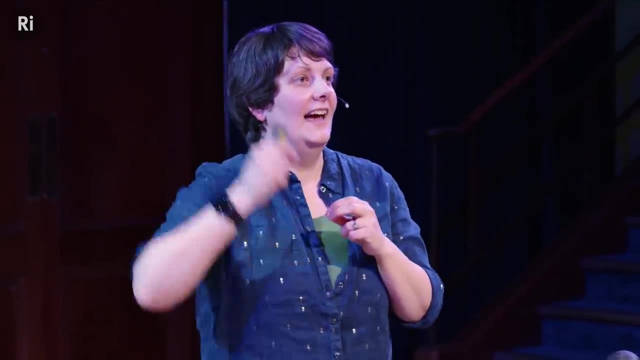 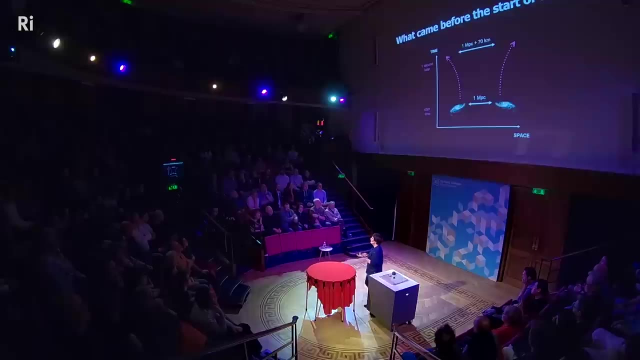 Can I sort of fly to the outer edges of the universe and go back on myself and come round again? Then another question is: how can I go round the Earth? And another question that people always ask is: what came before the start of time. 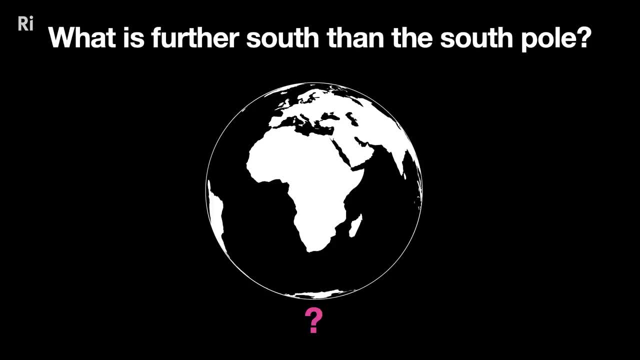 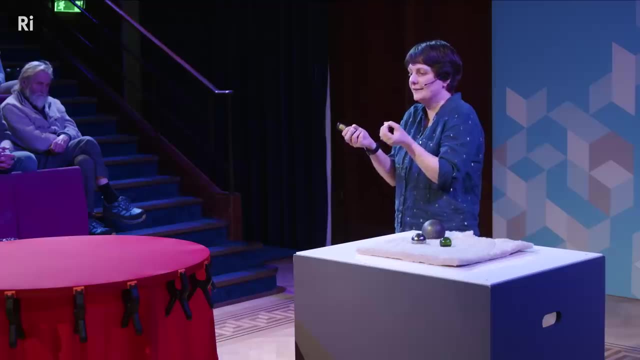 And this is like asking what is further south than the South Pole, Right? So if I rewind time in my picture of the sort of curved Earth, that's equivalent to saying: you know what happens when you get back to the South Pole And you know that on the Earth you know all people would come to. 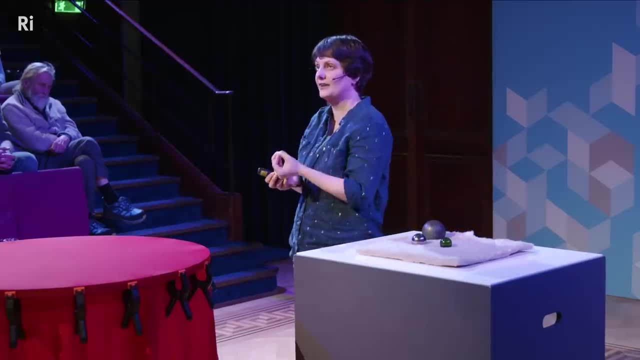 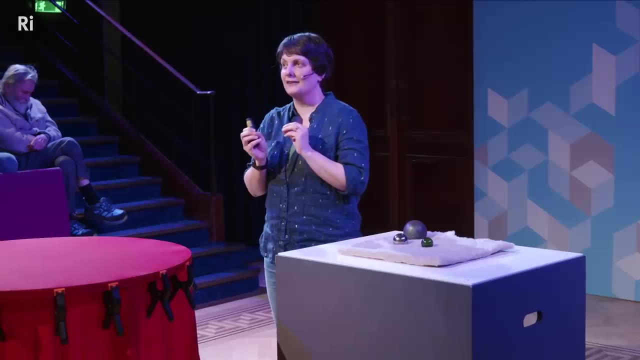 the South Pole. There'd be nowhere else for them to go. right, You can't go any further south than the South Pole. So of course you can start to think about what's going on in the Earth And you start asking questions about: well, somehow then you need to go off the surface of the Earth. 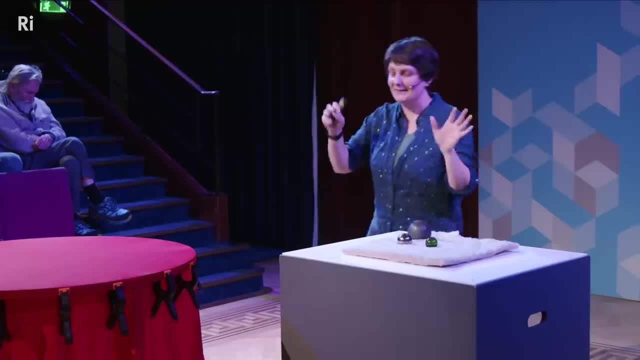 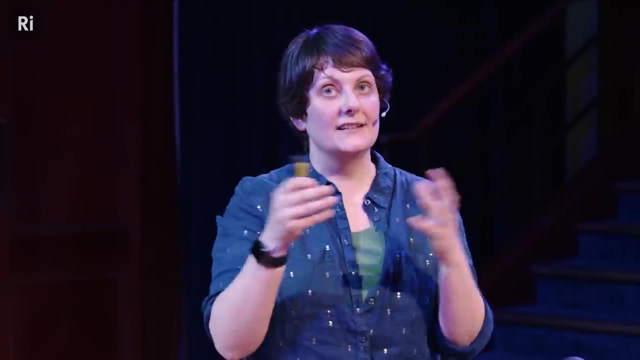 right, You need to go into a higher dimension. So then, you know that makes string theorists very happy. You know they think about higher dimensions and things like that. But you know, maybe that's the right question to be asking. right, You know, did this come from some higher? 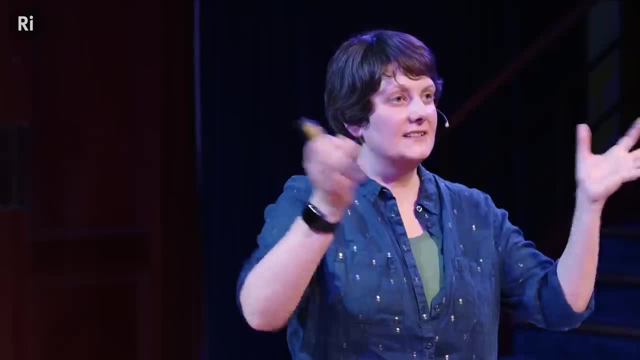 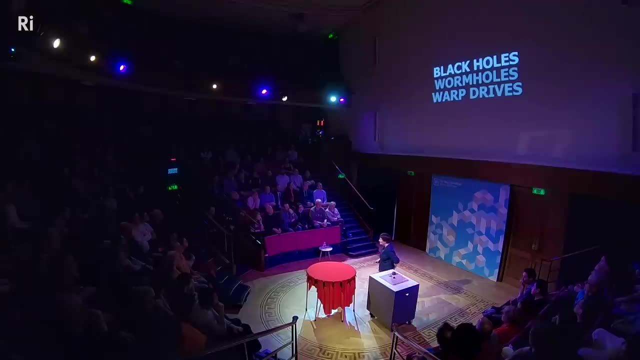 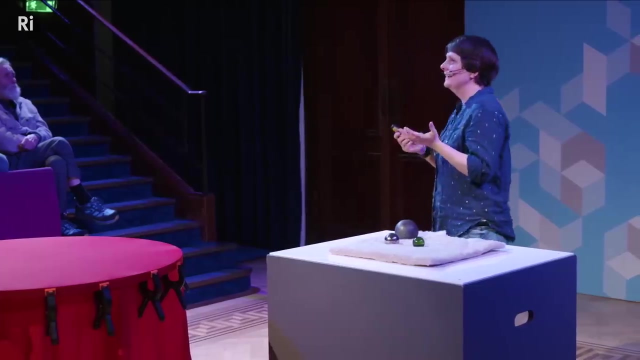 dimension. The two-dimensional surface of the Earth is somehow embedded in sort of three-dimensional space. Okay, So let me get on to black holes, Wormholes and warp drives, So starting with black holes. So I think the really interesting question to ask yourself. So I hope actually everyone knows what a black hole is. I kind of assume that if 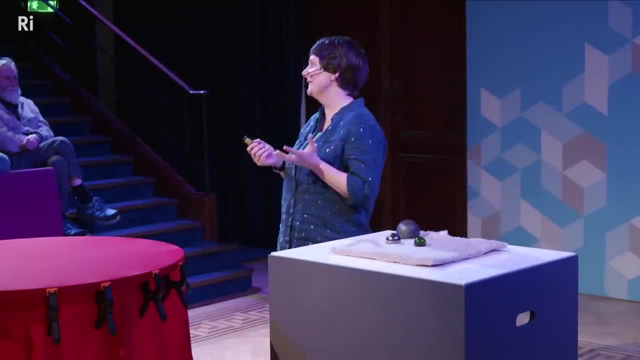 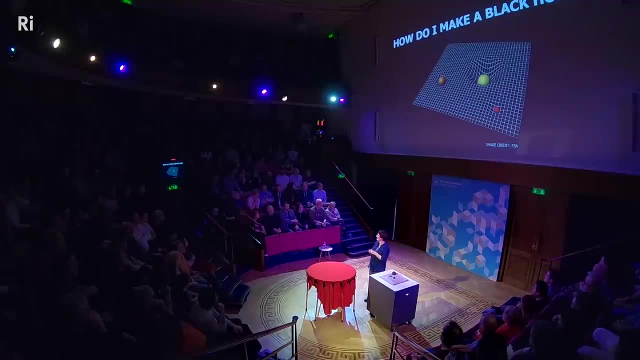 people sign up to talks like this, they've at least watched one science fiction film where there's a black hole in it. But maybe I shouldn't assume knowledge. Sorry, Star Trek. As long as people have watched Star Trek, you're definitely okay. You're going to really enjoy the end of the. 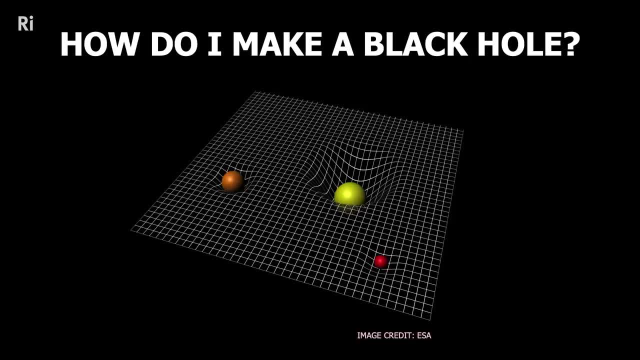 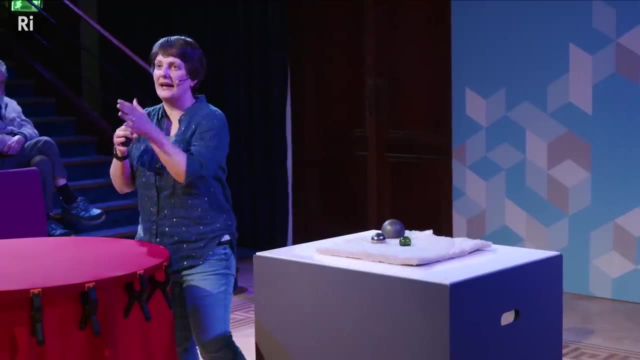 talk So. So, black holes, How do I make a black hole? So yeah, a black hole, as I say, the sort of definition of a black hole is a region of space and time that's somehow separated from the rest of the universe. So the idea is that you can't get out of a black hole. So there's some surface. 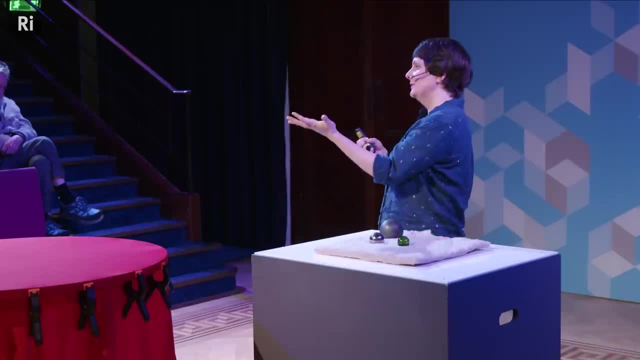 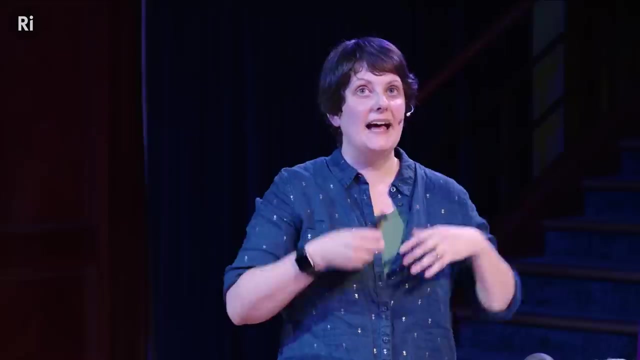 that once you've crossed it, you would need to travel faster than the speed of light to escape from it. And therefore you know- since, as far as we know, nothing can travel faster than the speed of light- everything gets trapped In a black hole. But the interesting question that I want to ask today is: how do I make a black? 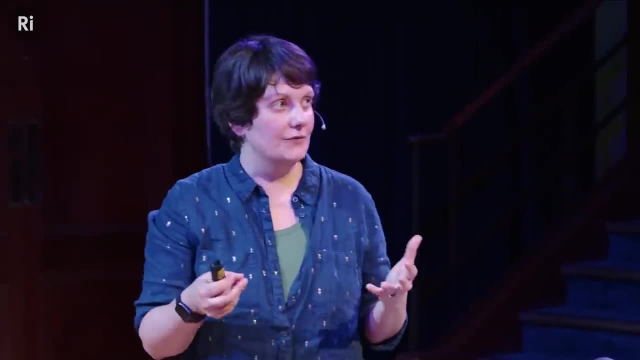 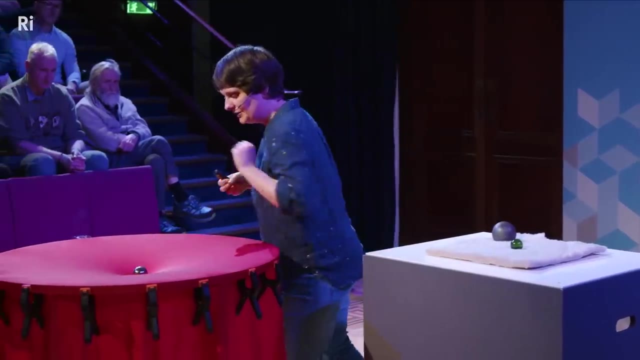 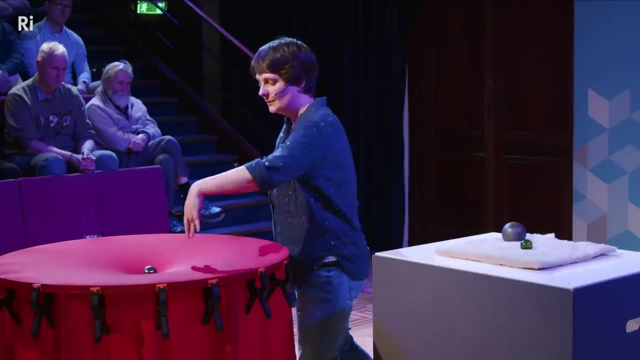 hole, Because that's really a question about you know, can one of these things really exist? How real is it? And so you know, I can now use again my little demonstration. What I want to do is I want to make this deeper right. So if I want things to get trapped in it somehow, I want this. 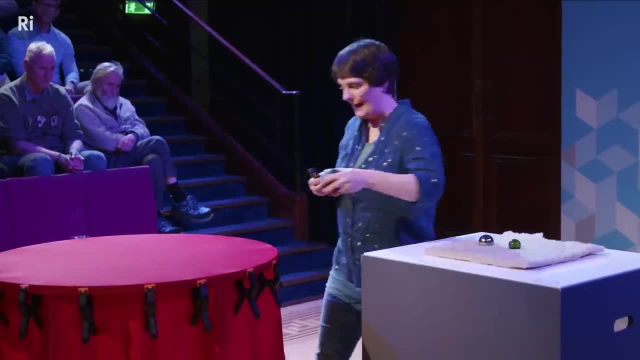 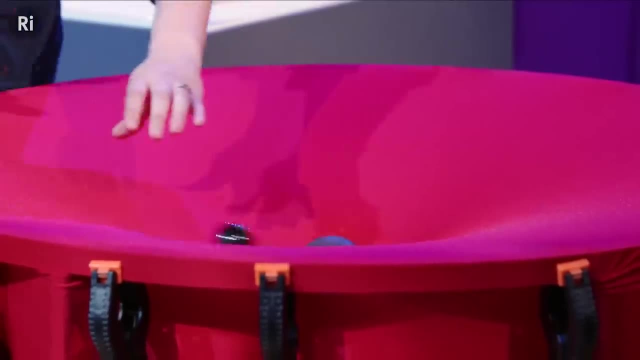 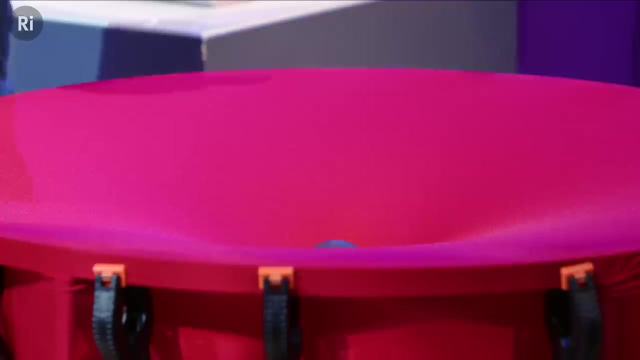 to make it go down So I can put my heavier object. And you see, it's getting deeper right. So it becomes more difficult for something to escape If I ooh. This is why I said I shouldn't be trusted with a demonstration. Ooh, It's really quite addictive. 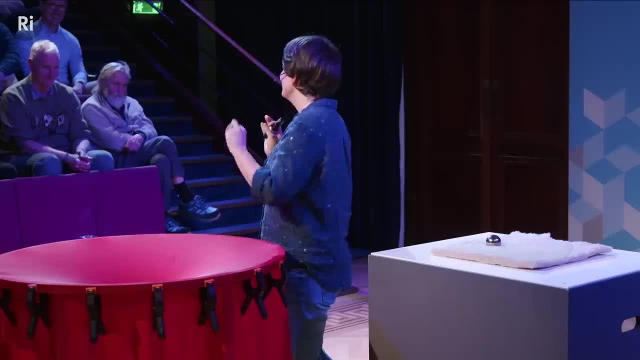 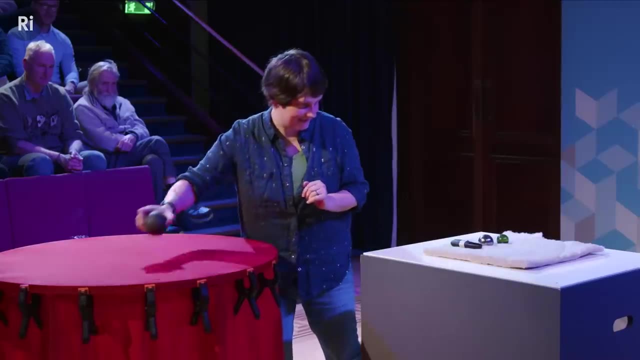 So they said that they will leave it outside once we finish the lecture and everyone can play with it. And I tell you, it is massively addictive, But I need something more right? So here we go. What have I got here? Ooh. 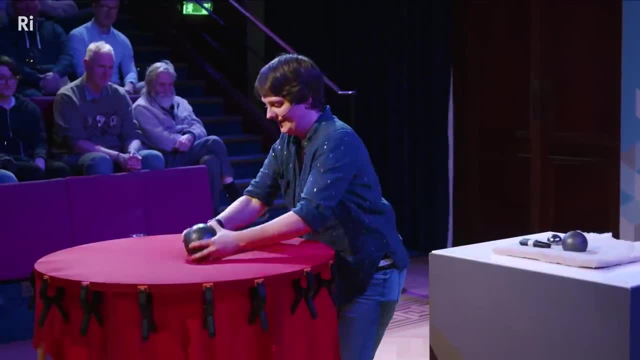 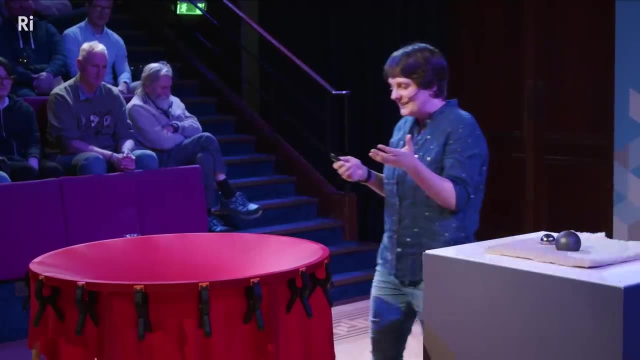 They said: two hands, Two hands, Bend your knees, Okay. So what I'm doing, right, what I'm doing, is putting more and more stuff into one place. So it's not enough. So, if you think about it, it's not. 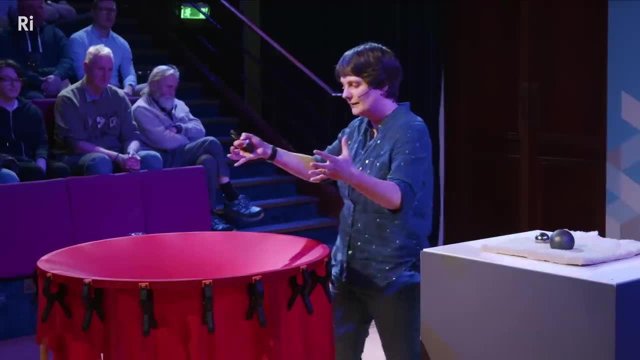 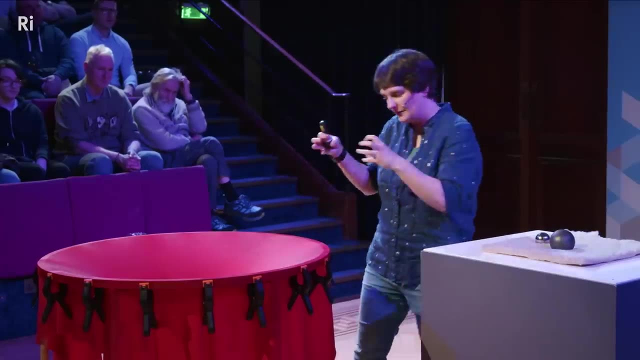 enough just to make the ball bigger. So obviously making it bigger isn't going to sort of give me this kind of tube that I'm really looking for. I need to somehow contract this stuff into a small space. So I need something that's very big, I need something that's very small, I need something that's 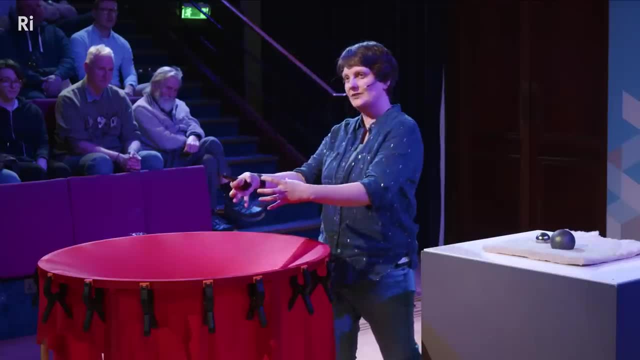 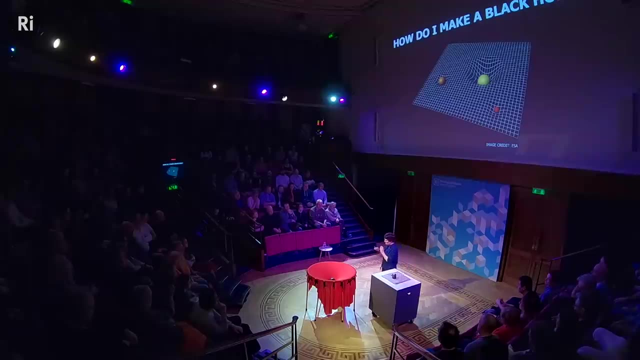 very dense. So this ball is very dense. So having a ball of the same size but a lower weight wouldn't work right. So this is the thing we have to do. So actually, what we have to do is we have to get all. 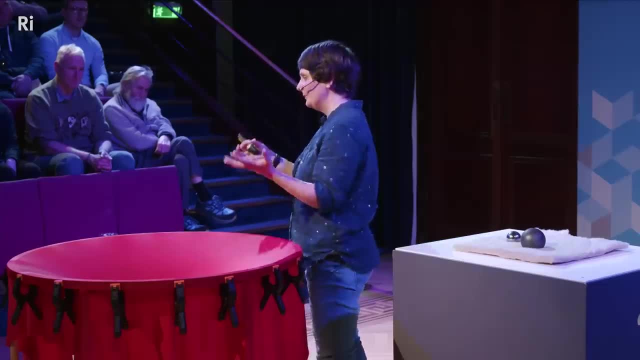 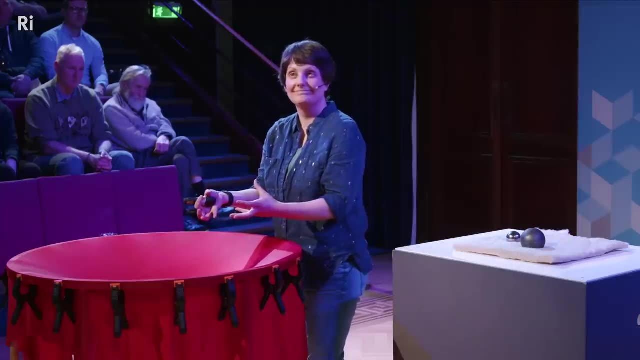 the mass that's in the sun, so all the matter that makes up our sun, and we have to sort of squash it into a region that's only a kilometer across, Right? So a kilometer is like I don't know here. 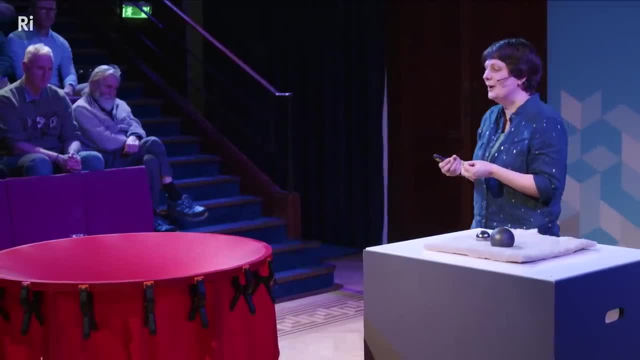 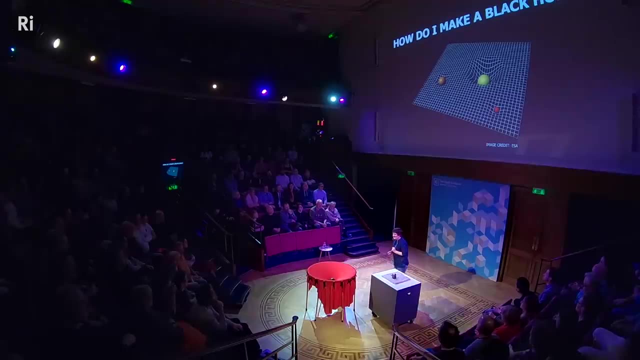 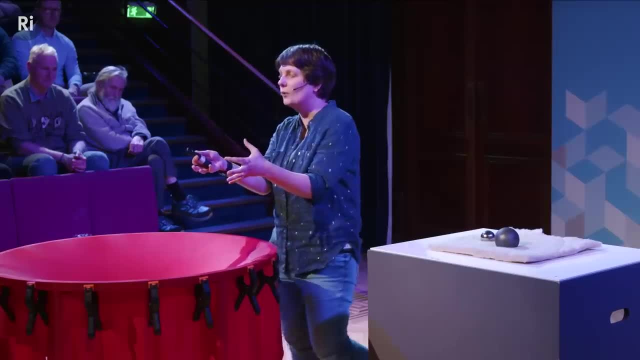 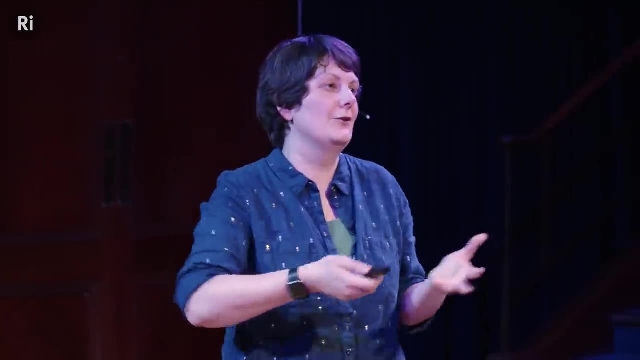 is sort of compact the sun into a region that's very small And so on the face of it. initially people thought black holes sounded crazy because they said, well, you know how did that happen. That seems like it would be really hard to do, right, Like how do you get the sun and squash it? 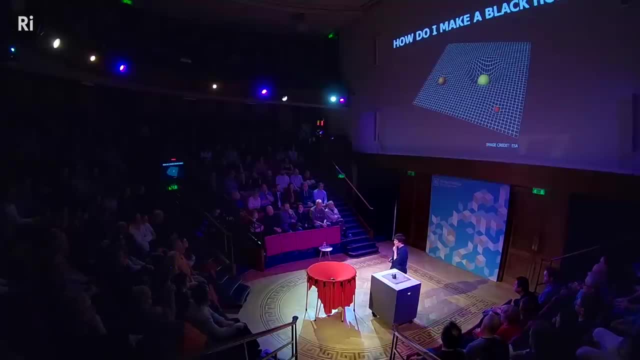 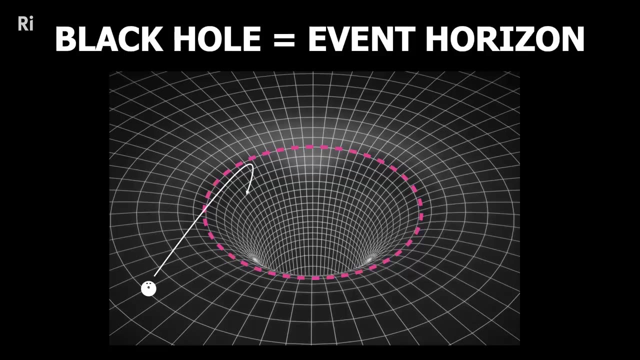 So initially people thought that black holes were just a mathematical curiosity. So yeah, So, as I said, they have. So actually the point I wanted to make- I was going to do it with slides as well, but then they made me do it with this. 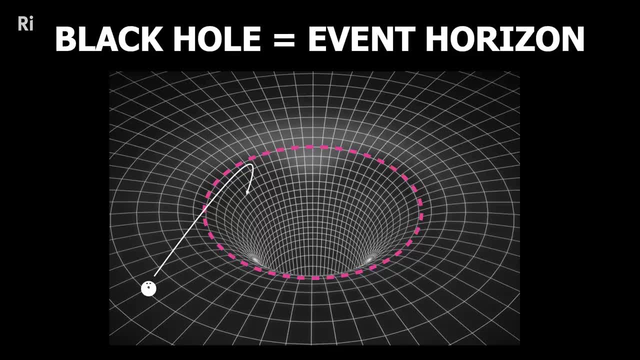 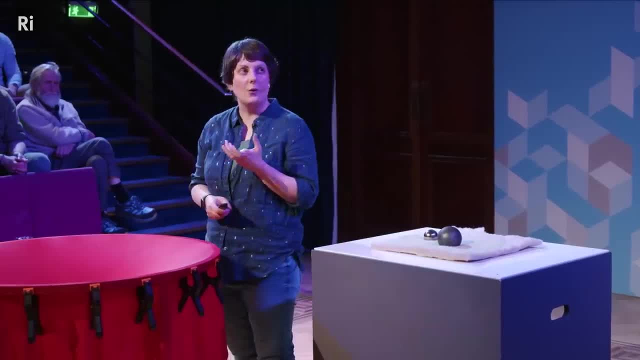 So what I wanted to say is that actually, technically speaking, black holes are this event horizon. So it's quite interesting, We don't actually describe black holes by what they're made of. So if you think all the other things that we have in astrophysics, like a star or a planet, 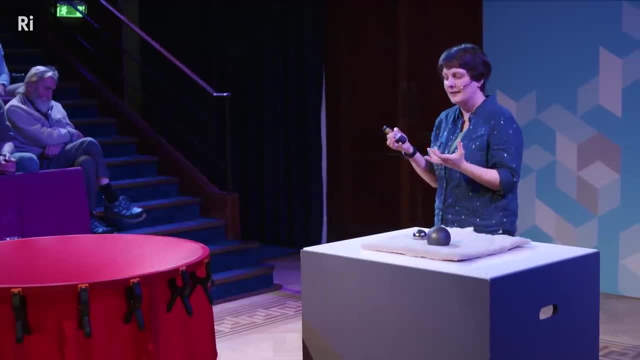 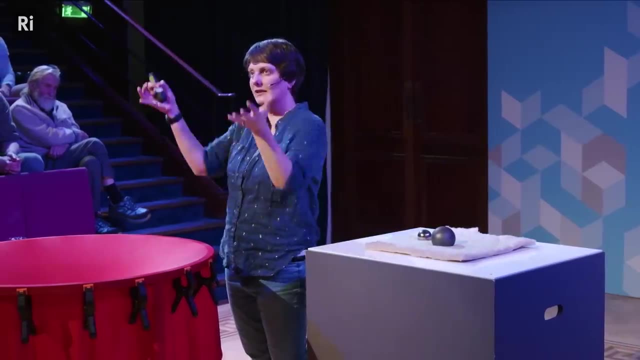 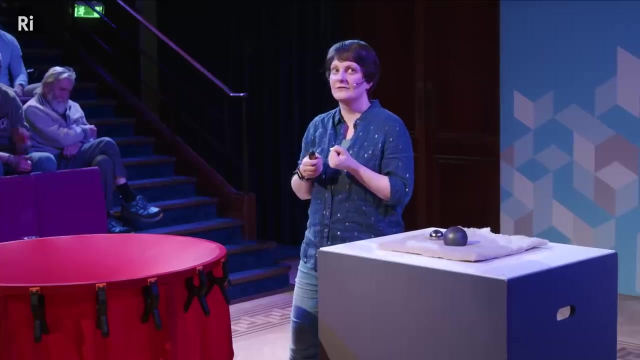 we generally describe. We don't actually describe them by what they're made of, But with black holes we actually don't do that. We actually define them as just being this surface beyond which nothing can escape, And one of the reasons that we do this is because we really can't know what's in them. So there's. 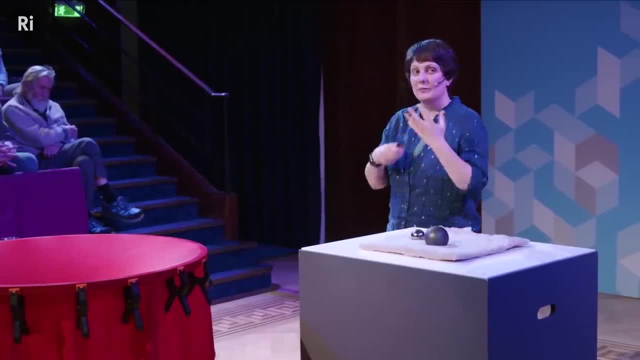 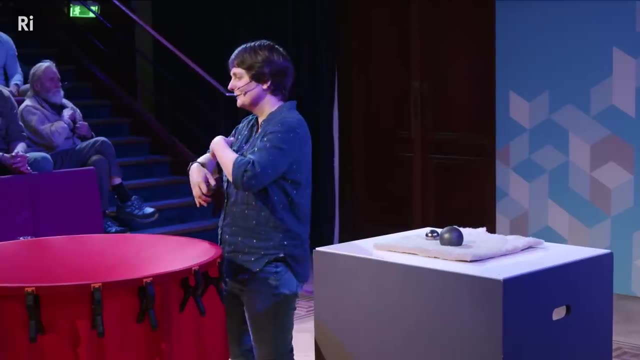 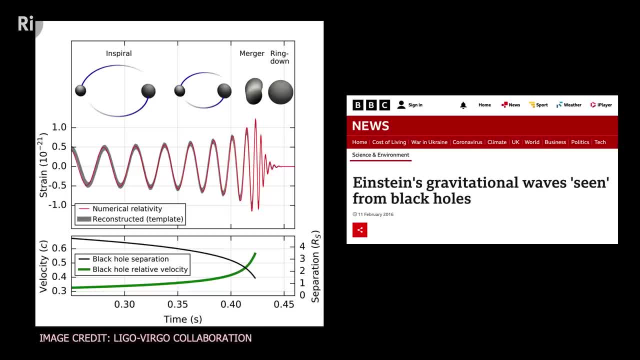